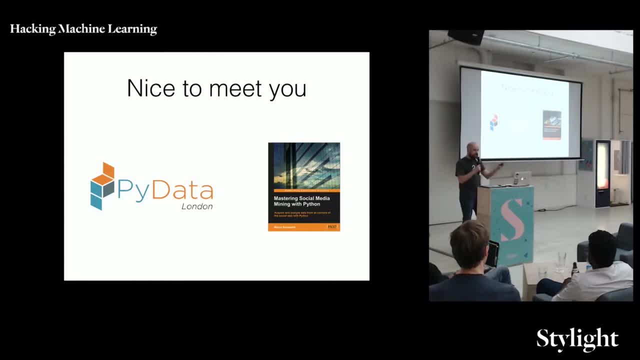 and conference. so we run a monthly meetup kind of similar setting: couple of talks, nice people, few beers and so on- And we also run our annual conference. it was back in May, also in London And on the right side you see some work that I've done. this was a book published last. 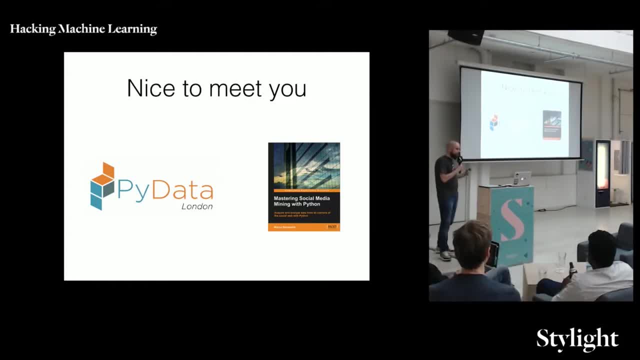 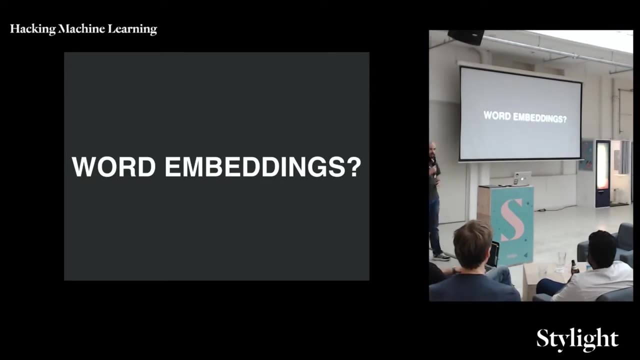 year on data mining for social media. So the job title is data scientist, whatever that means, and in particular I try to focus on text analytics. So word embeddings. the structure of the talk will be kind of an informal introduction on word embeddings: first what they are, what we want from them, and then a little bit of 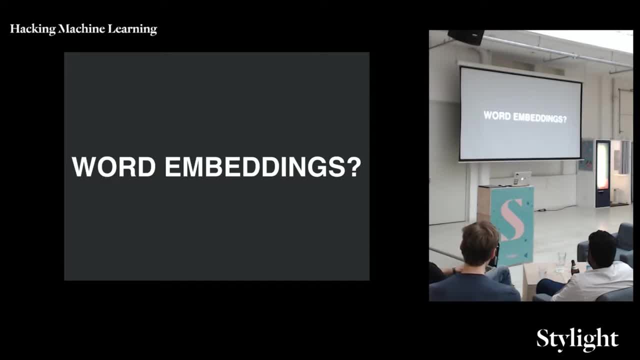 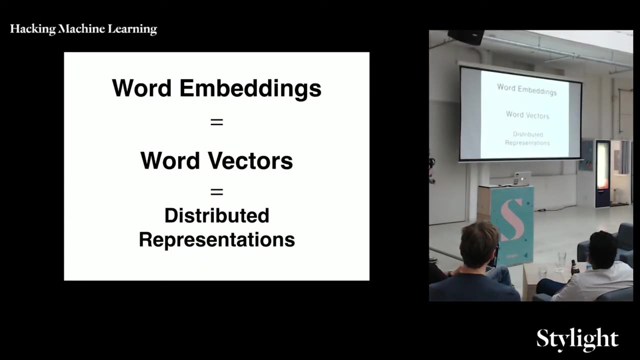 theory, but not too much. this is meant to be really an introduction, so if there are machine learning experts in the room, maybe you will not learn too much on the machine learning side, But it's more on the linguistic intuition And then a bit of Python at the end. 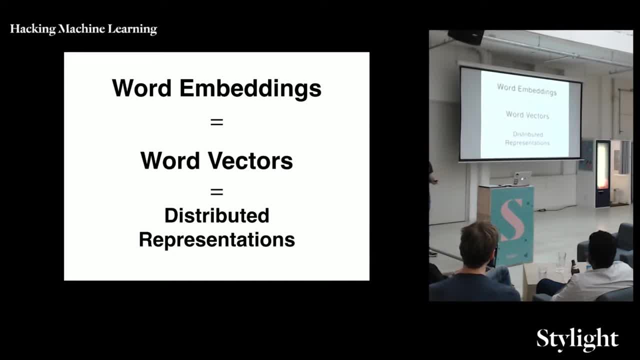 So terminology word embeddings are vectors that represent words. So what you see here, they're all synonyms, word embeddings, word vectors, also semantic vectors, because these vectors capture the semantics of words And also distributed representations is another way to call word embeddings, because the meaning 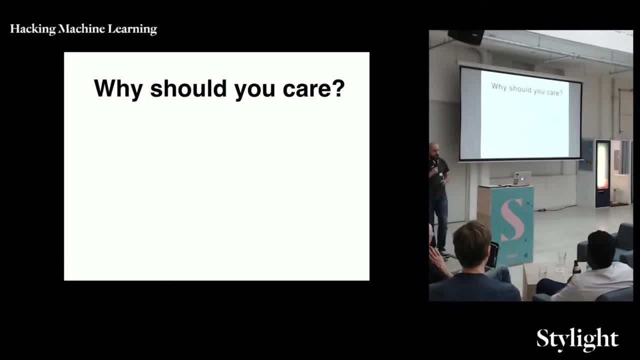 of a word is distributed. It's distributed across many dimensions. So why is this important? Well, in data mining, the way you represent your data is crucial for the success of your application, And in text mining that's the same story. So word embeddings are really interesting ways of representing text. 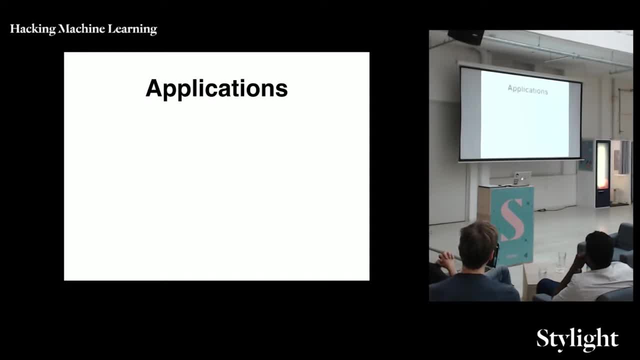 In terms of applications. where are these word embeddings useful? Really? anything about text analytics is fair ground to try out some word embeddings. I just mentioned a few bullet points here, but that's not an exhaustive list. So classification or tagging, assigning classes to documents, recommendation systems, search. 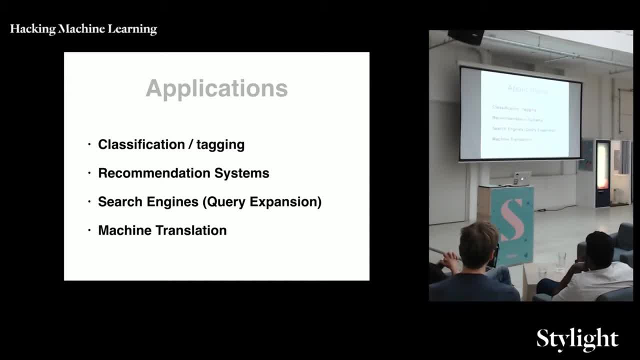 engines, So you type in your query and then the search engine can expand your query and understand what you're trying to search. And then a bit more difficult machine translation, So going from English to any other language. These are all applications where word embeddings have been applied successfully. 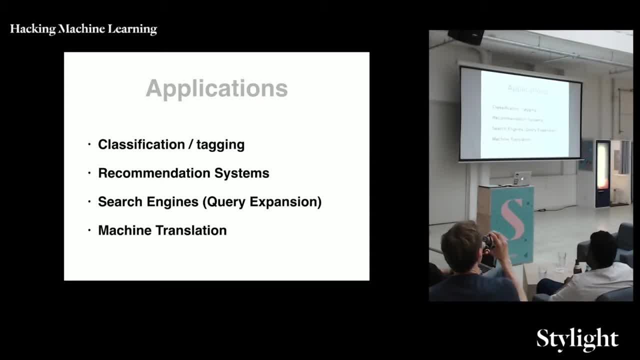 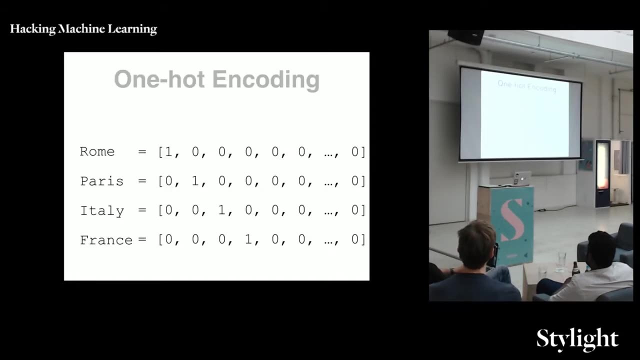 So you can use them in a lot of different ways, And there are many more, So really everything about text analytics is a fair game. I want to start with a couple of ways of representing text, So the first one is the classic one-hot encoding. 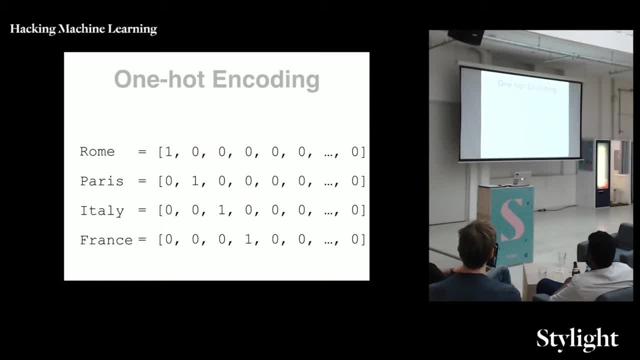 So in one-hot encoding you have lots of vectors representing words And you see you have zeros everywhere And then you have only one bit being hot at a time And this is good to represent categorically. You can use it to represent words as well. 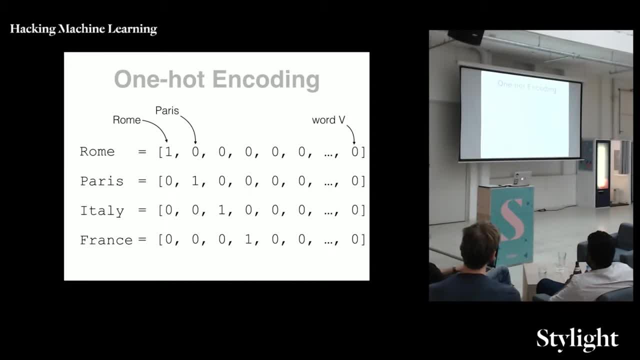 So essentially every dimension that you have there is representing a word. So first bit for Rome, second bit for Paris, and so on until the last word. There is a problem here. We are basically having a lot of dimensions, So the size of your vocabulary potentially is huge. 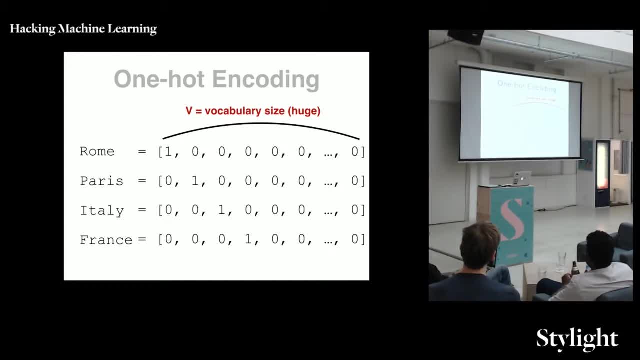 So there's a dimensionality problem And also we don't have any notion of similarity. Right, There's a similarity between these vectors because these vectors don't have any dimension in common, Right? So you cannot calculate easily any kind of similarity. 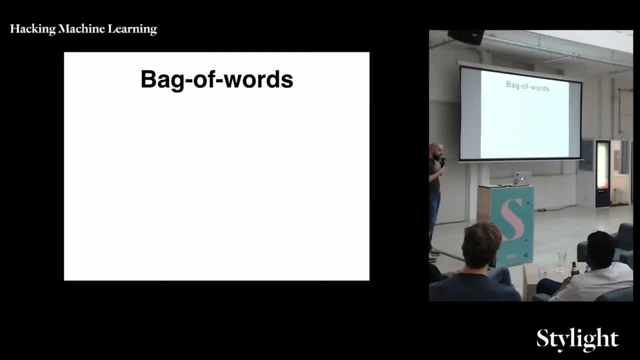 Another approach to represent text is the popular bag of words. This is used usually to represent documents. So with documents you also have vectors, for example, And again each dimension is essentially representing a single word. This could be you know how many times you see the word Paris in document one. 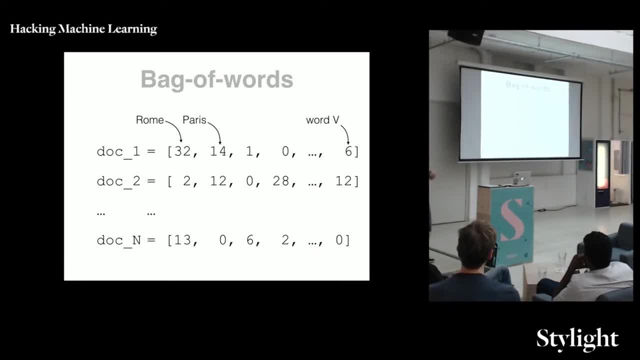 That's 14.. How many times you see the word Rome? That's 32.. That's a row count. You could normalize it in many other ways, But again you have a big number of dimensions And at least you start having some notion of similarity, because you might have some. 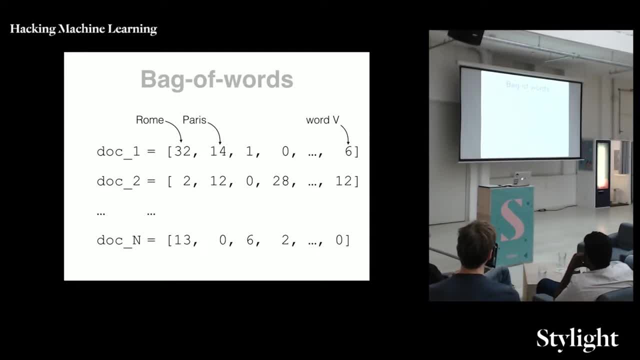 dimensions in common here, So you can compute similarity between vectors. Okay, Now moving on with word embeddings. So word embeddings are also vectors. The example is kind of made up just to showcase a couple of aspects of word embeddings. So what we want from word embeddings, we want the number of dimensions to be much, much. 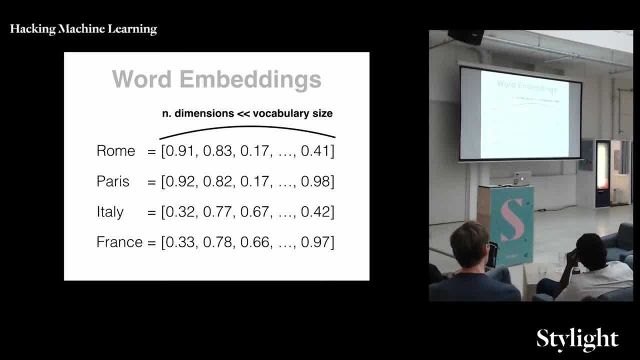 smaller than the vocabulary size. And then we want to capture some ideas of similarity. So, for example, Rome and Paris are somehow similar. Okay, They're both cities, they're both in Europe, they're both capitals, they are both nice places to visit. 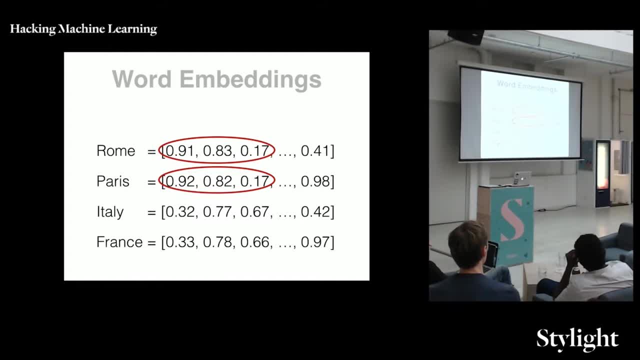 So a few dimensions. you see the numbers are kind of close to each other. Similarly, Italy and France. they're both countries, they're both in Europe, good wine, good food and so on. So you want to capture the similarity with some dimensions. 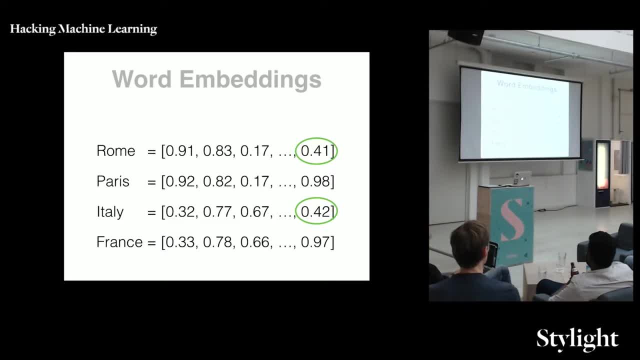 Also Rome and Italy and Paris with France. they are kind of similar to each other in the sense that there is a semantic relationship. So Rome is the capital of Italy and Paris is the capital of France. And this semantic relationship, you want it to be captured as well by some of the dimensions. 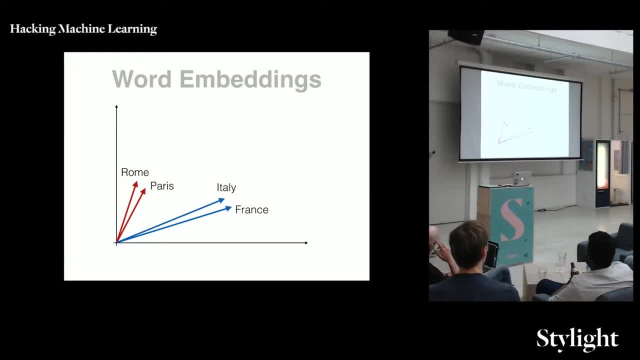 Once you go into kind of pictures, if you try to picture it, you see Rome and Paris as vectors. They're close to each other because they're similar. Italy and France as well. they're close to each other because they're similar. 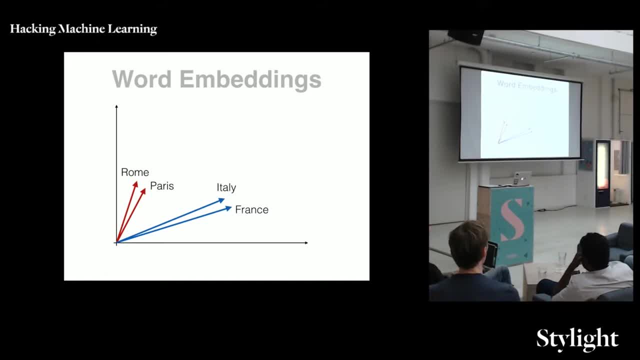 And you see, there's almost this direction from Rome to Italy and from Paris, Okay, To France, which is representing the relationship of being capital of. And that's the nice aspect, with word embeddings, So you can do vector arithmetics. You start with a vector for Paris. 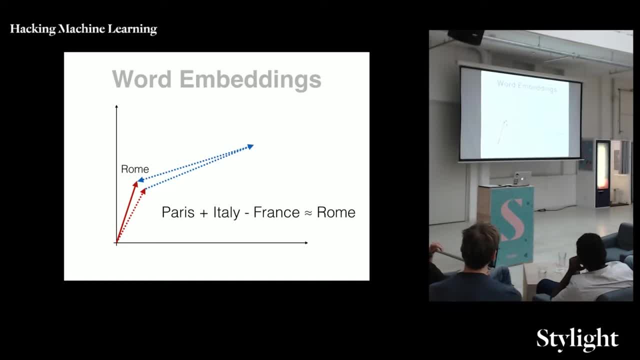 You add the vector for Italy and you remove the vector for France, You will end up with a vector which is very, very close to the vector for Rome. Okay, So you can perform this analogy task. Maybe you've seen before The king minus man plus woman, equal queen. 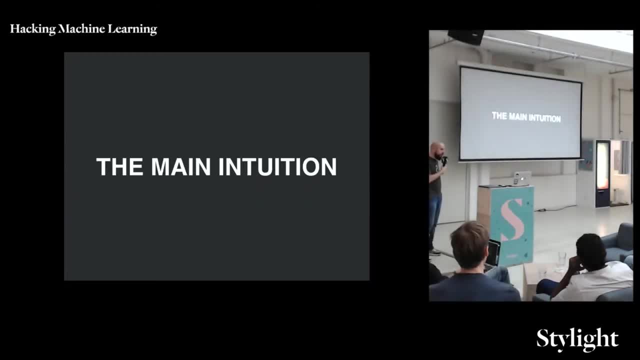 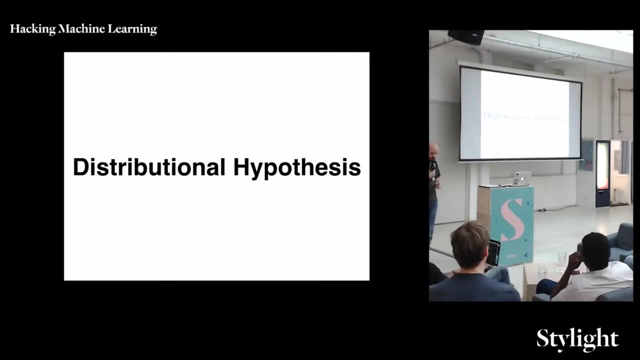 That's also an analogy. So we don't have vectors, yet We have language. So what is the main linguistic intuition behind these models? That's called the distributional hypothesis, And this is nothing new. Okay, This goes back to the 50s. 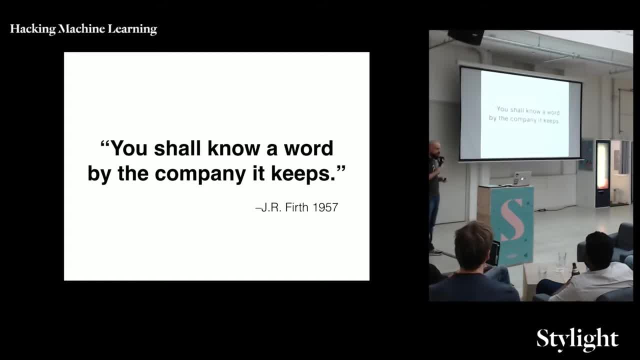 And, in particular, you find the reference. usually every talk about word embedding is a reference in this particular course, Because if you found that word, you were in a position of position. It has nothing to do with language, And so if you find that word in a language, it's not a reference to the language that. 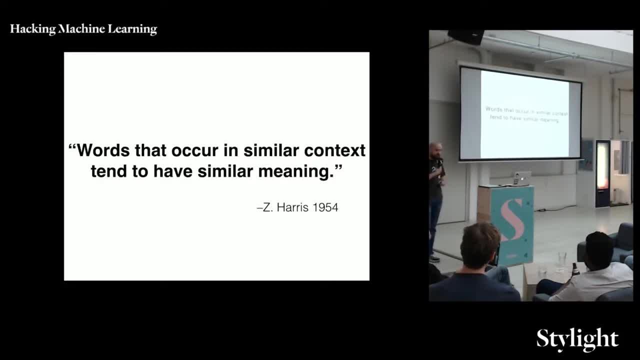 exists in this particular case. Okay, So I'll share a couple more examples. I'll show you the gracias. For example, in the operative code, You should know, a word by the company Equips, by the Spanish professor of linguistics 1957.. 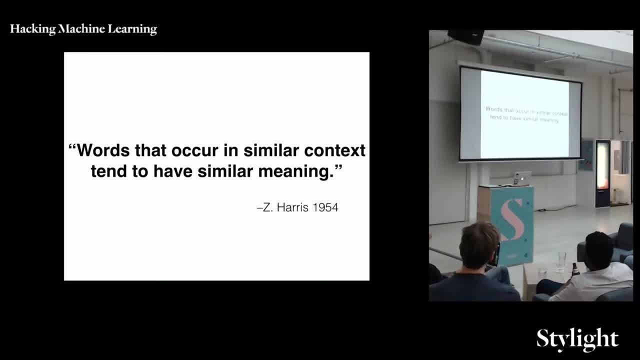 And maybe it sounds a little bit too intellectual, So there is another one from a couple of years earlier, which is probably more clear: straightforward Words that are called in similar contexts tend to have similar meaning. Okay, So that's as simple as it is. 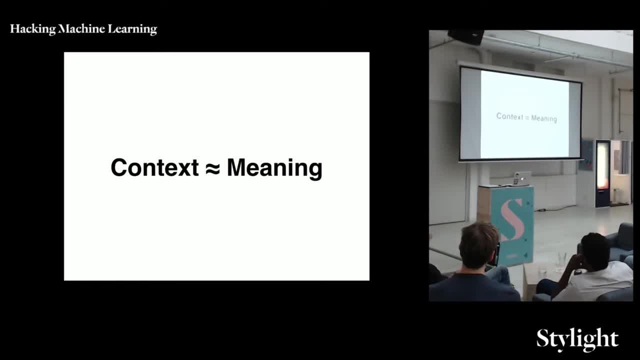 We can use the context. So what's going on around a particular word? To apply the context, approximate the meaning of the word itself, And I want to give you an example. So this is a sentence. I enjoyed eating some pizza at the restaurant. 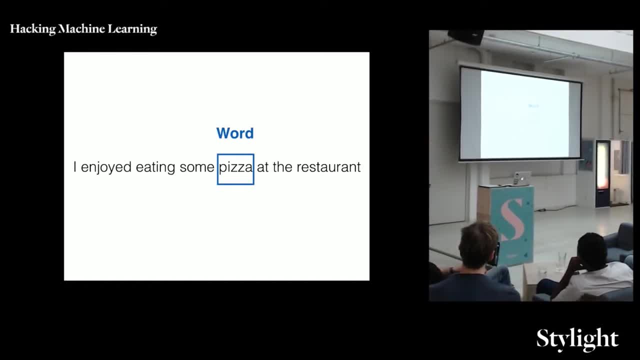 We focus on what's important, So that's the focus word. the word pizza And everything else is the company keeps. So that's the context of our word And essentially we can approximate the meaning of the word pizza just looking at the context. 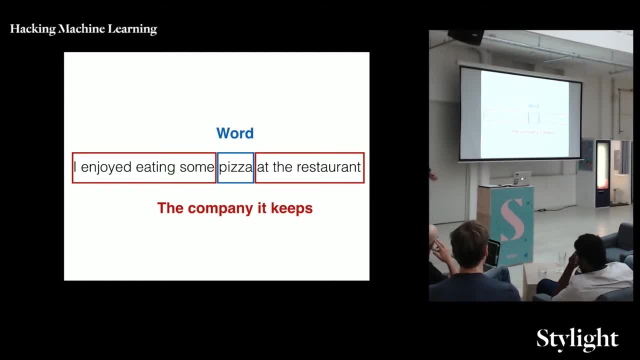 So pizza is something that we eat, Pizza is something that we have at the restaurant, Pizza is something that we enjoy. And then you scale it up on thousands of sentences. You see how the word pizza is used in the sentences And once you aggregate, you end up. 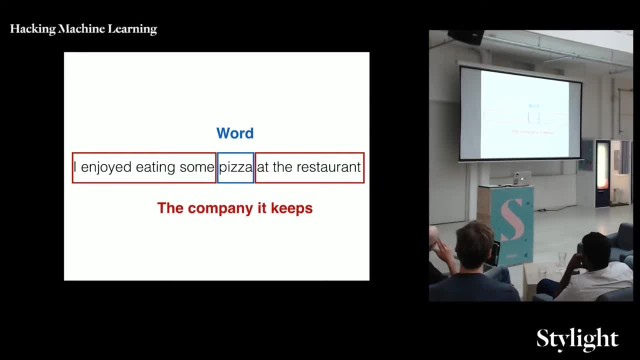 with the true, deep meaning of the word pizza. And now I give you a counter example. So you have two different sentences: I enjoyed eating some pizza at the restaurant And I enjoyed eating some Weisswurst. Did I spell it right? 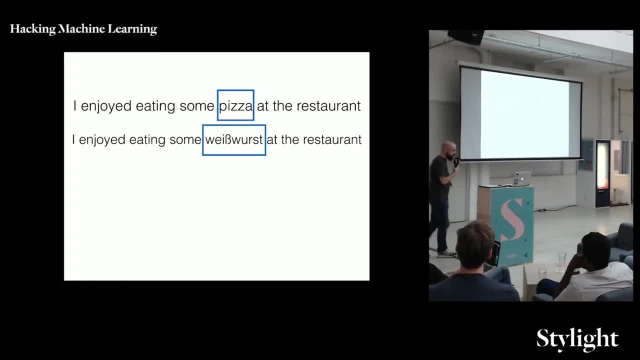 Yeah, OK, so these are two different focus words And maybe you already see where this is going. So we have the same context, According to what I told you so far. same context, same meaning. So for some people maybe having pizza or Weisswurst. 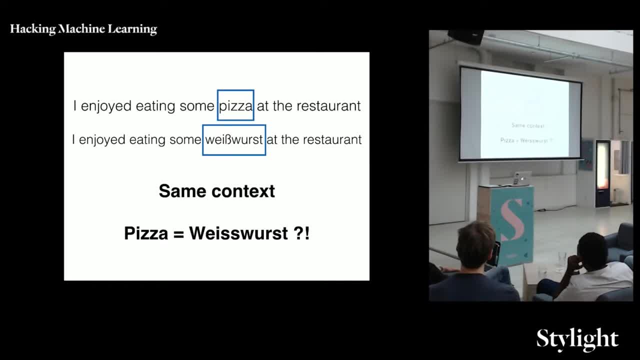 is the same thing. For me, this is kind of outrageous. Don't blame me, Blame the data. That's what the data look like. That's what the model is going to pick up. So this is just to have a bit of fun with a simple example. 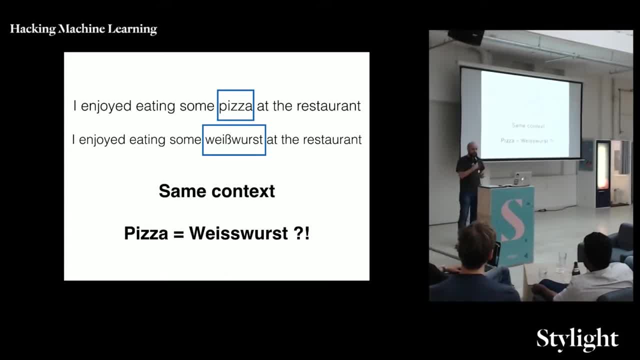 But really it opens for a discussion on data quality. Your model is only going to be as good as your data And possibly about ethics, because language is going to be biased. It will pick up the biases from your culture And your model is going to pick up the biases from your language. 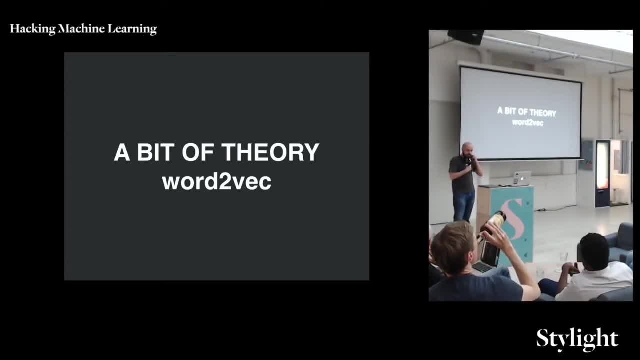 OK, now, moving on with a bit of theory, I'm going to mention in particular the Word2vec family of algorithms. So word embeddings are a family And Word2vec is kind of a family within the family, And Word2vec is what started all the interest a few years ago. 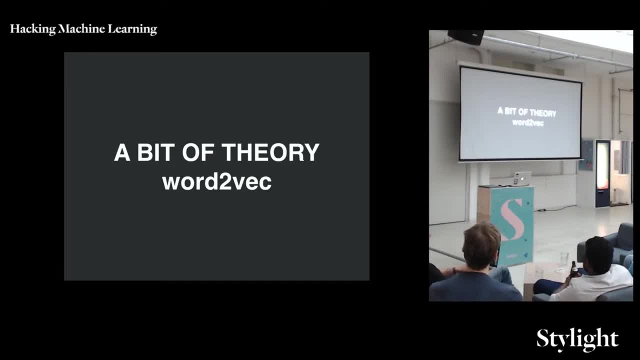 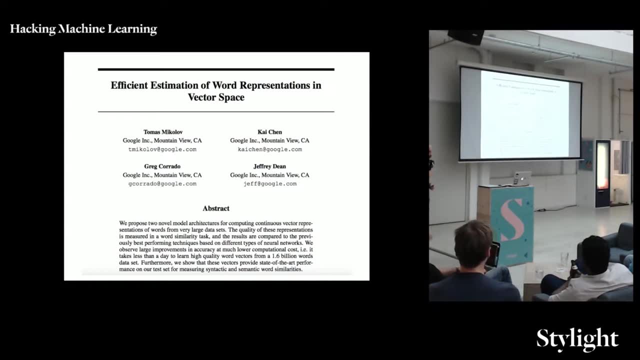 around 2013, on these word embeddings and on doing arithmetics with words. So this is work that has been done at Google. So Thomas, So Mikolov and colleagues published a couple of papers in 2013,. Efficient Estimation of Word Representations. 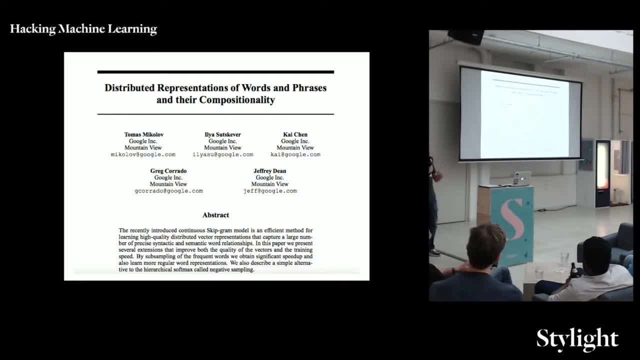 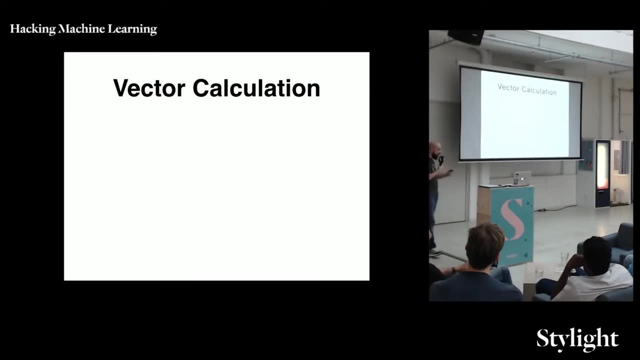 in Vector Space and also Distributed Representation of Word Phrases and Their Compositionality And the concepts from these papers. they ended up in what we know today as Word2vec. So about the vector calculations? So how do we get vector from language? 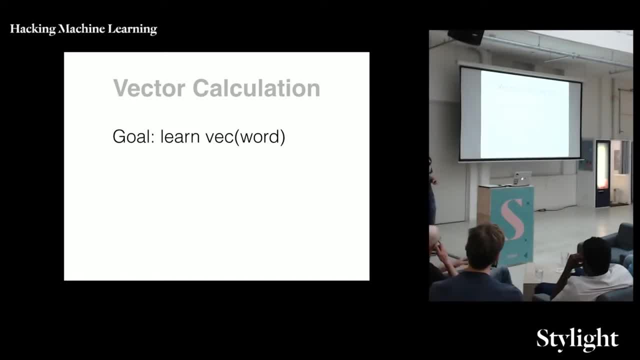 The goal, then, is learn vectors that represent words, And we're going to look at things from a distance, from the high level. So, first step, choose an objective function. Second step, initialize randomly our vectors And third step, run stochastic gradient descent. 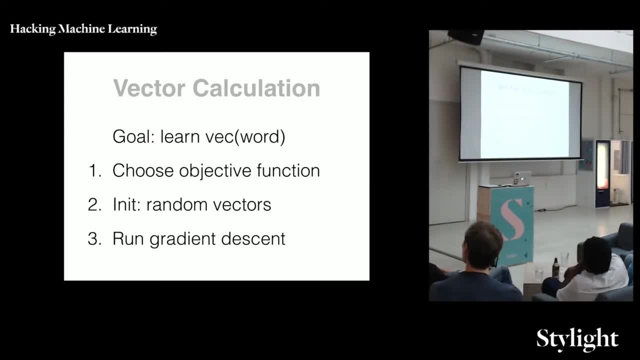 until you end up with the vectors. And if you've done some machine learning before, maybe you've seen the same approach applied to many other different contexts. So from a distance sometimes machine learning looks kind of everything the same. So what's interesting here is really: 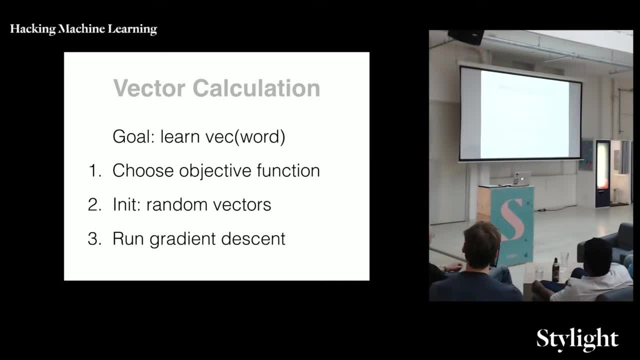 what's going on with the objective function? So the objective function is something that we want to maximize, and we call it the gain function, or something that we want to minimize, And in that case we would call it a loss function. And I go back to the example. 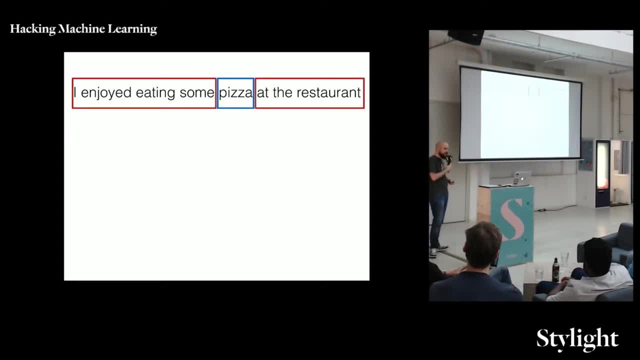 So we have the sentence, The focus word is pizza and that's our context. So the objective function in this case is we want to maximize the likelihood of observing the context given the focus word. In other words, we're going to end up. 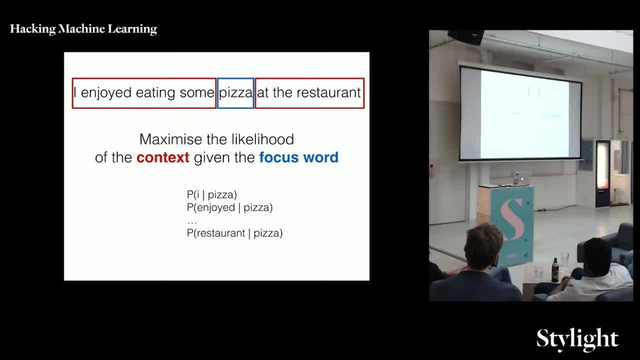 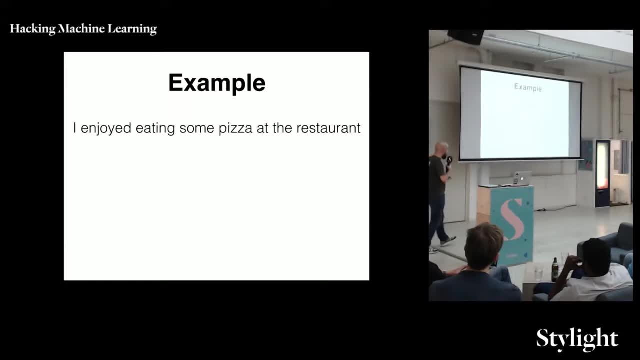 with a bunch of probabilities that look like this. So, probability of observing a context word given the focus word. Let me look at the example with a few more details. So we have our sentence as before, We have our focus word And we need to iterate over all the context words. 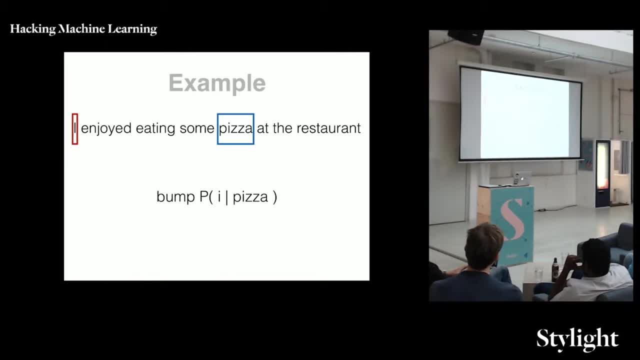 So we start from the beginning of the sentence. We see the word I, given that the focus word is pizza, So we bump up the probability of I given pizza. And then we move on. We see the word enjoyed given pizza And we bump up the probability of enjoy given pizza. 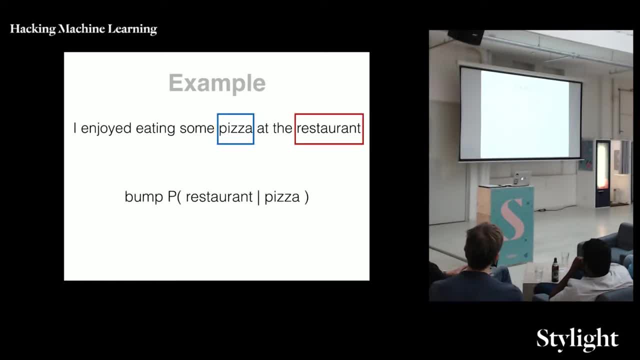 We see the word eating and we bump out the probability, And then again, and again, And again, until the end of the sentence. Once we reach the end of the sentence, we move on to the next focus word And we repeat the process. 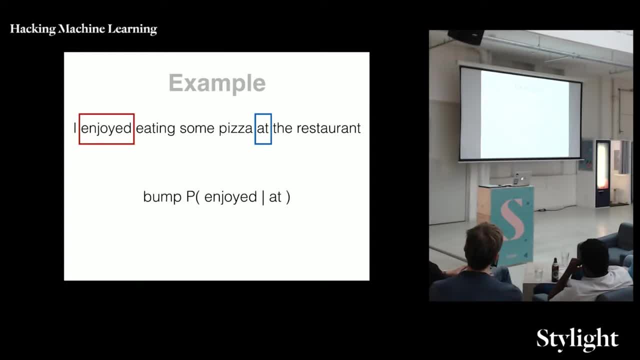 So, starting from the beginning, you see, I given the word ate, Bump up the probability. You see, enjoyed, Bump up the probability, And then you see where this is going. So, essentially, two nested for loops, And then the core, the heart of the matter. 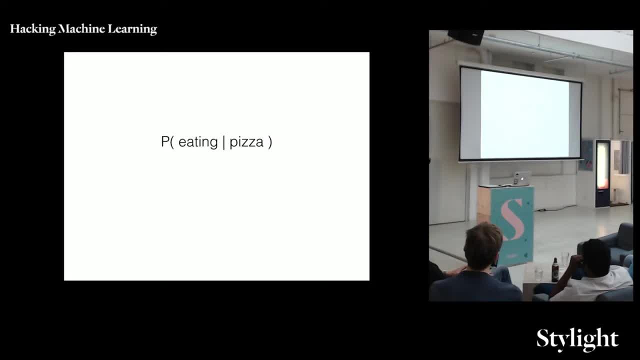 is bumping up this condition. So the word pizza is the initialbooing to the additional probabilities. And I keep saying bump up the probabilities, But we haven't defined any probability yet. So what's the probability of eating pizza? Question mark. 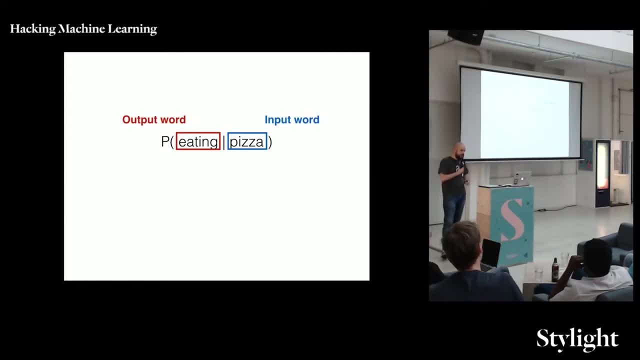 We can generalize: We called the condition the word pizza, in this case the focus word also input word And we call the context word also output word And we want this to have more than one conditional World And we want to have one conditional world. 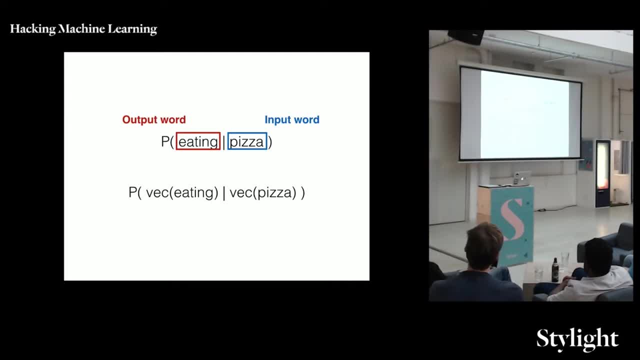 this probabilities to be dependent on the vectors. So we kind of rephrase the probability as probability between vectors. So using this notion of input and output, we can rephrase it as observing or bumping up the probability of the output vector given the input vector. and again we we've been 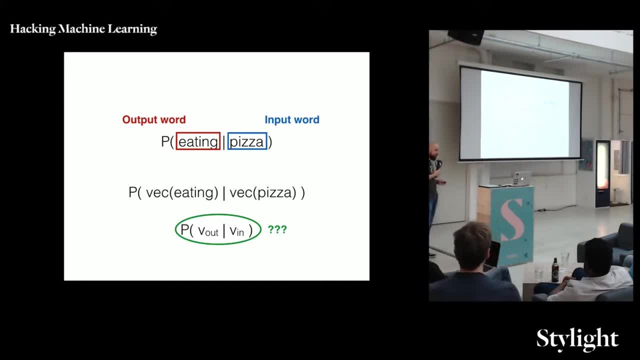 rephrasing, but we haven't defined any probability yet. So we have this probability defined as vectors. Ideally we want the probability to be high if the vectors are similar. So first idea that comes to mind, use, you know, cosine similarity or other notions of a vector similarity. that's a fair. 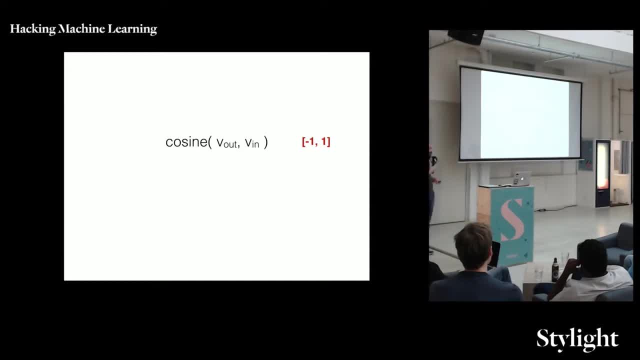 intuition. There's a problem here. cosine similarity is not a probability right. it's a number between minus 1 and 1.. Next idea: take the cosine similarity and throw it into a softmax function. The softmax is used in many machine learning approaches. It gives you as: 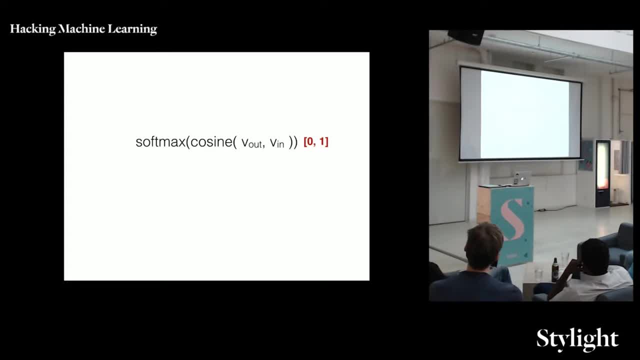 output a number between 0 and 1.. So it looks like a probability and it turns out it's also has a probabilistic interpretation. If you want a formula, that's the formula. So the probability between vectors is essentially defined as the exponential of the cosine normalized over the sum across all the 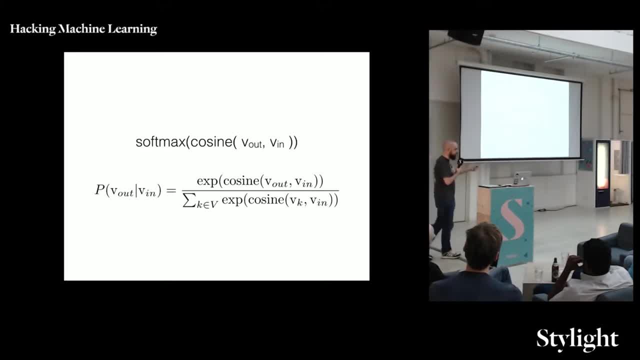 vocabulary. So all the exponentials for all the cosine similarities Between output world and input world. Okay, if you have done some machine learning before, this is kind of maybe nothing new. If you're new to it, don't worry too much about the, the formula. Try to look at things from a distance. So 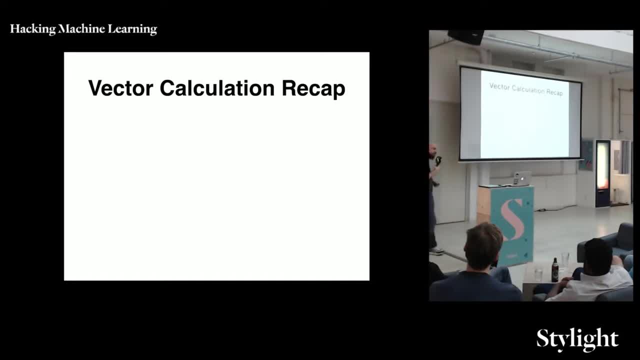 just to recap this idea of computing vectors. what we've been doing, we've been learning word vectors using stochastic gradient descent on the softmax probability as defined before. So here you have all the ingredients that you need to apply this algorithm if you want to look it up. If the theory was not enough, there is more. It turned out, you can also learn. 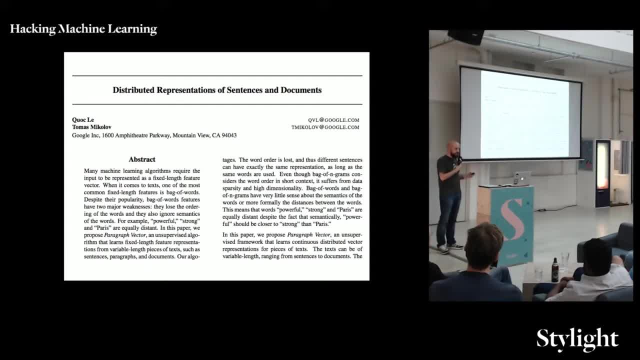 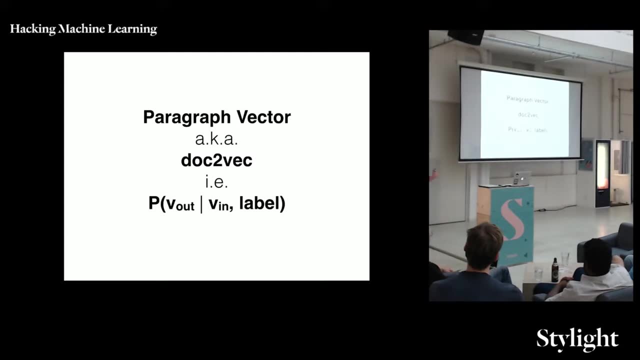 not only vectors for representing sentences, but also for representing- sorry, not only for representing words, but also for representing sentences or documents. And that is a follow-up work, also from Google, and in that paper they call this algorithm paragraph vector and, just as a reference to word2vec, they also call it doc2vec, And what we have here is pretty much the. 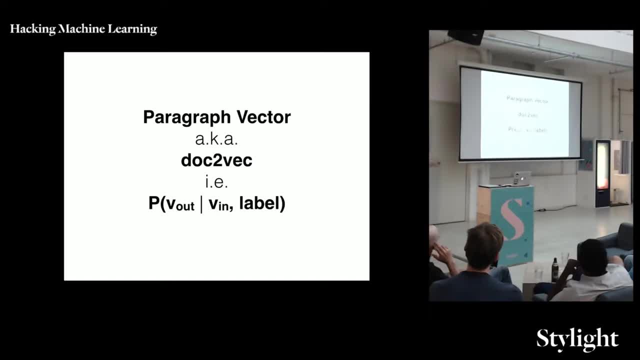 same. the only difference is how we define the probability between vectors. We also attach a label as a condition, and the label could be a sentence ID, a document ID, anything kind of ID that you use to group all your words into a particular paragraph. Okay, and that's, that's really. 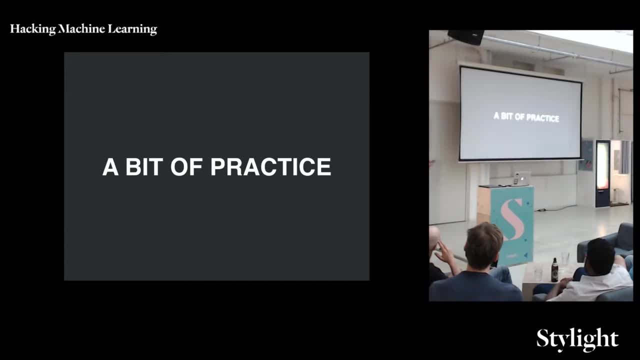 enough for the theory. Of course I haven't given you too many details, but that's kind of the overall idea. Now moving on with the practice. So word2vec became popular because it was an academic success on one side, and also because Google released the software as open source. So there's a C library for 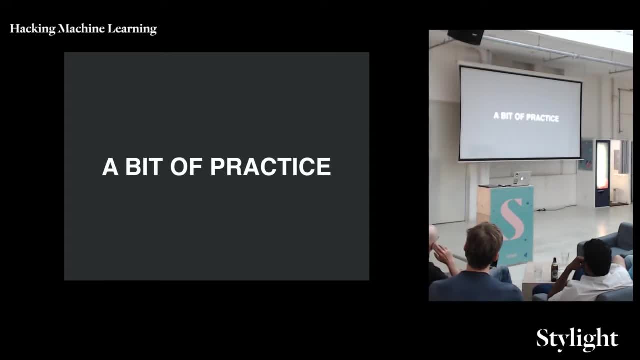 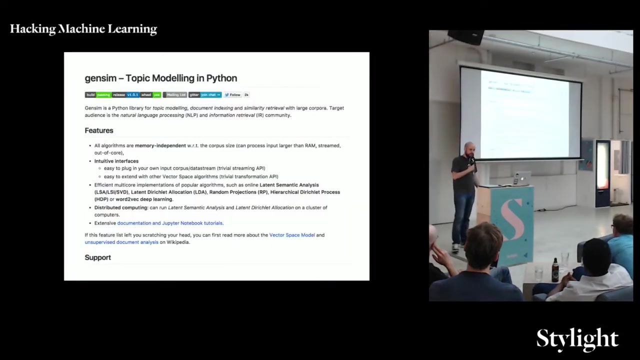 training your vectors, And they also released the binary form for some vectors that were pre-trained on some Google News corpus- so billions of words that you can use. so essentially, you kill the training times to zero if you reuse those vectors. We're doing Python anyway. so let's look into Python For Python. we. 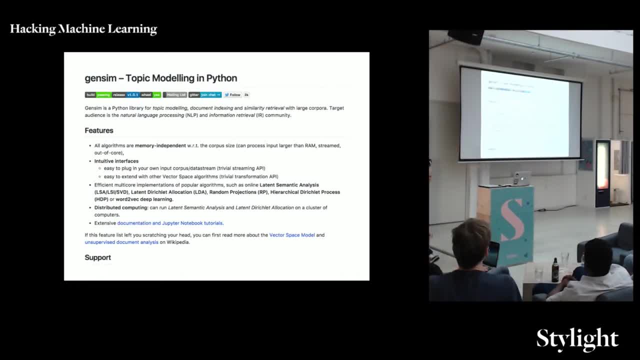 have this library gensim. One line for them is a topic: modeling for humans. So what they do is they implement a bunch of NLP text analytics algorithms and they stick a nice interface, easy to use interface on top of it. And when they implemented the 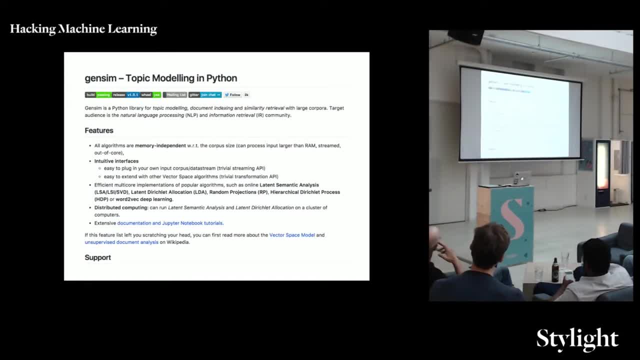 word2vec algorithms. it turned out the gensim implementation in Python was faster than the original C implementation in Google, So that's how they got a lot of traction. So Python faster than C, That's a lot of work. There's a lot of Cython and crazy NumPy kind of optimization, so that's how it was. 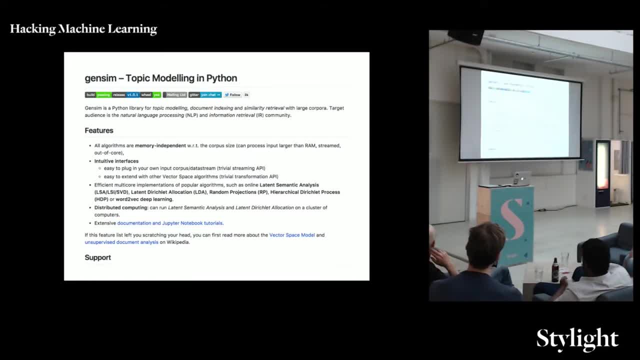 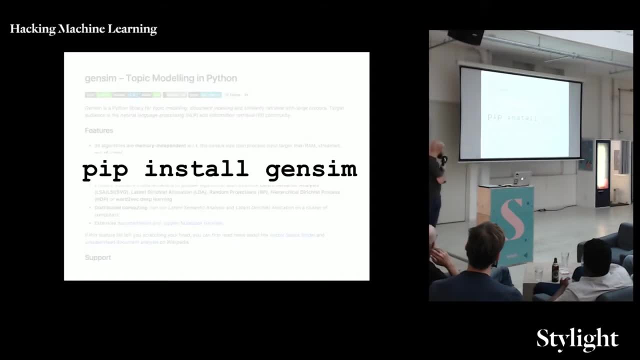 possible. Anyway, as users of the library, we only look at the interface, which is Python. so very, very simple, easy to use. Okay, so pip, install gensim or, if you prefer, conda install gensim. if you, if you do data science, you should go with. 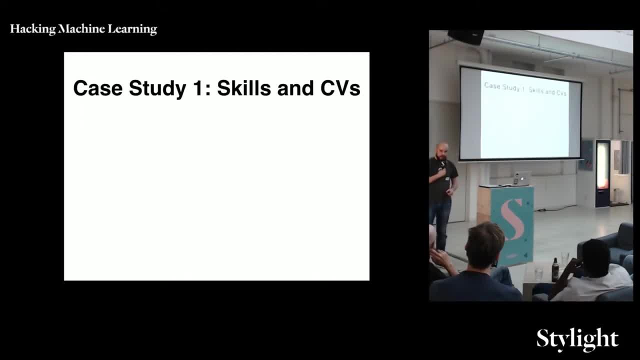 conda and you're good to go, And I want to give you a couple of examples of how it works. So what? we this, this vector. so there's some work that they did with a previous client of mine. they have a recruitment platform, so you upload your. 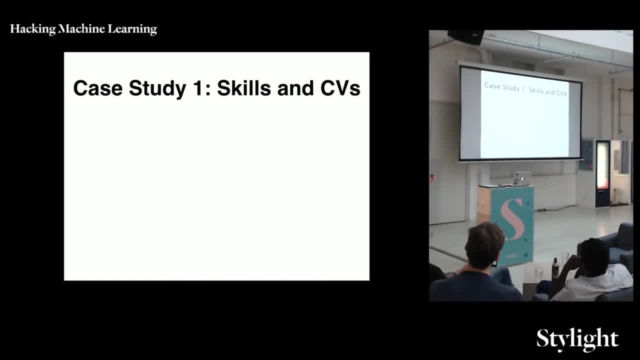 CV. Companies upload job specifications and then the machine learning magic in the middle that tries to match the best people for for the job. Essentially we were looking at CVS and the skills describing a CV. So we did a little bit of a pilot to see if word embeddings 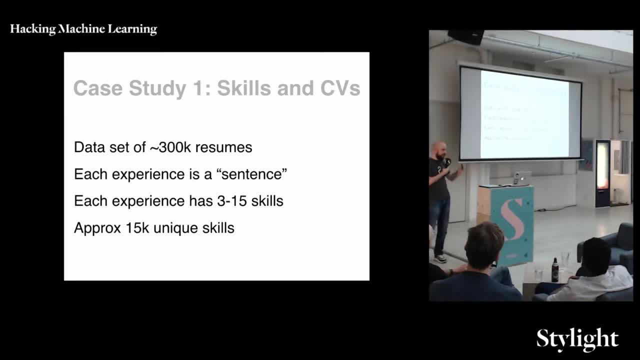 could be useful. We had a data set of 300,000 CVs. Each CV has a bunch of experiences and we treat each experience as a sentence And each experience has a bunch of skills associated to it. Approximately, we had a vocabulary. 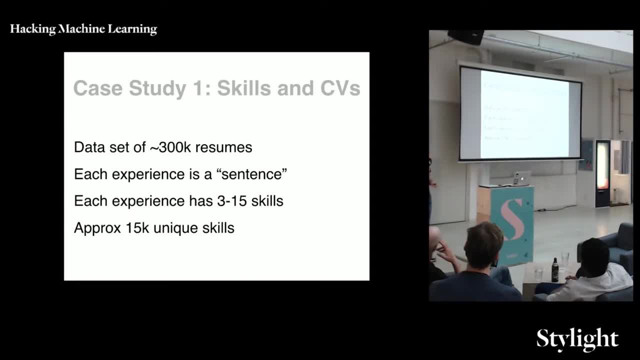 of 15,000 unique skills, so unique words, so not a huge data set, And that's the ginseng part that you need. So essentially you import the class. You have your data set somewhere in JSON, CSV, any kind of format. 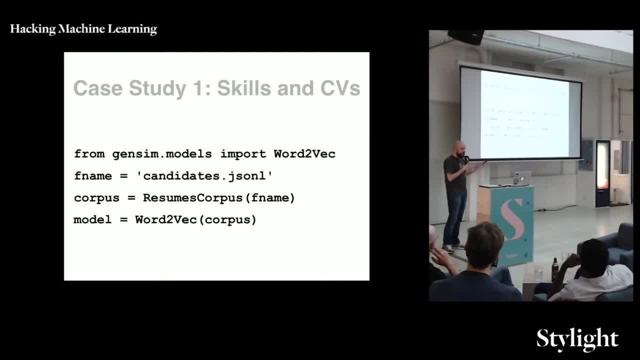 It doesn't really matter. The custom part that you need to implement is your corpus reader. So the third line, the class, will be probably a generator that yields one experience at a time. You don't need to load the whole data set in memory. 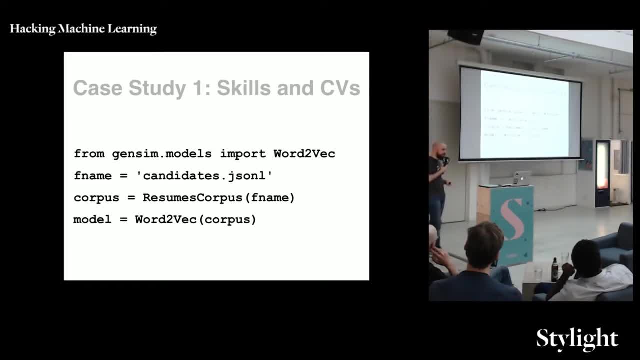 only one item, one sentence, one experience, in our case- at a time, And then you pass the generator to the Word Chef class to load the model. And there are a few extra arguments there that I'm kind of hiding the details to keep it simple. 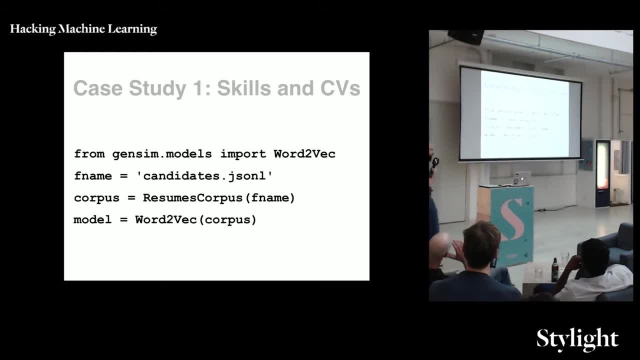 You can choose a couple of options. You can choose the number of dimensions for the vectors and so on. So you end up with a bunch of vectors and you can look at vector similarities. So, for example, we have the Word Chef and we look at similar words. 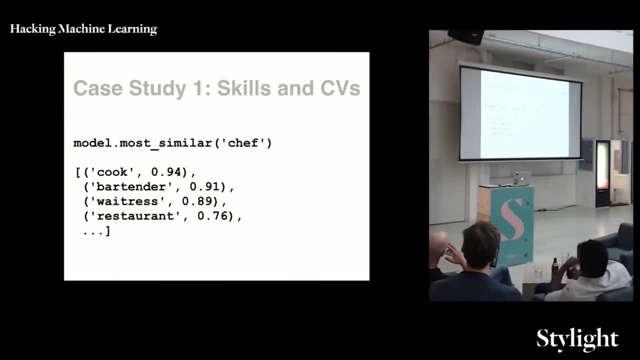 And the first one is the most similar one to chef cook. So they are synonyms And that's perfectly fine. And then, if you carry on, you see bartender, waitress, restaurant and other related words. These are not really synonyms, but they. 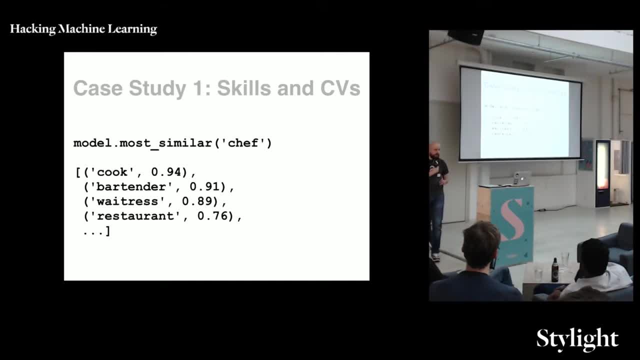 are similar in the sense that they kind of belong together. See restaurant business or the food industry, if you prefer. So it makes sense. The Word Chef also has another meaning. If you are an infrastructure engineer or DevOps, chef might be one of the tools that you use. 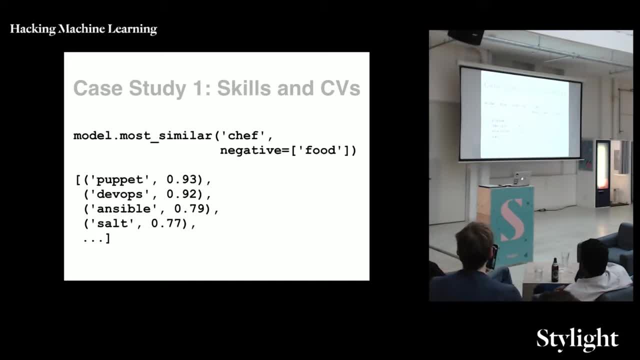 It's the name of a library. So this is the magic: with Word Vectors You can do arithmetic. So take the vector for chef, remove the vector for food and you end up with a vector which is very, very similar to Puppet Ansible Salt. 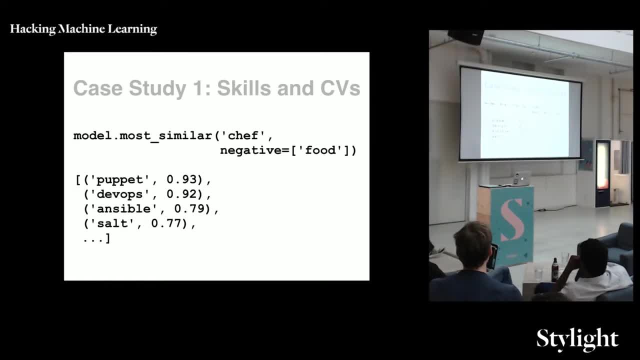 These are all libraries in the DevOps kind of space. So essentially the model was able to pick up these nuances of the language. So the main meaning, The main meaning of the word chef is, let's say, the obvious one with the restaurant business. 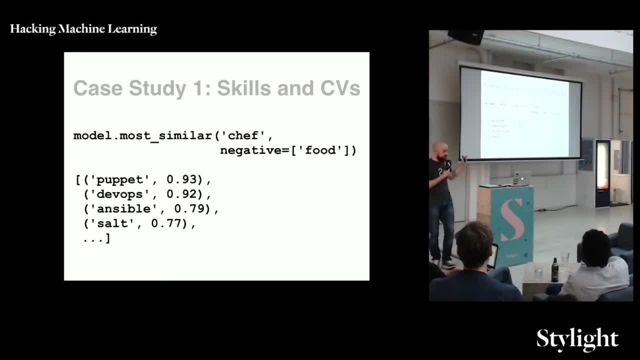 And then also doing this arithmetic, we were able to observe these kind of similarities. So the model was very, very useful for the data exploration phase. really understanding our data was crucial, And also we put it in production later for query expansion and query suggestion. 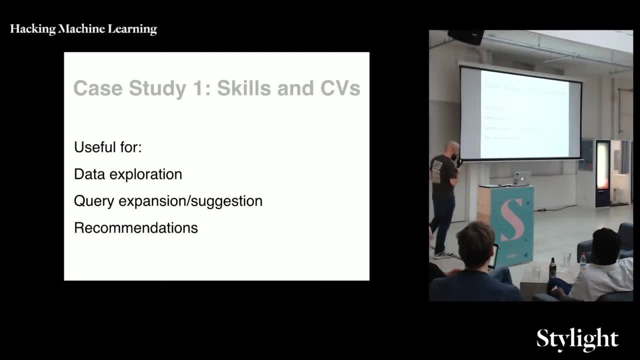 So again, you type in your job spec as a company and you see what kind of skills belong together. And finally for recommendations. So the algorithm for recommending people and jobs was influenced by the embeddings. Now, on a lighter note, different kind of use case. 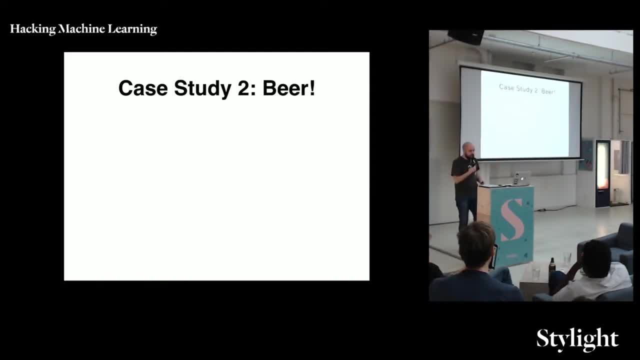 Bit of a side project for me. I like data, I like Python, I like beer, So why not put in everything together? So there's a data set for research of beer reviews- around 3 million documents- And all the beers are classified according to the beer style. 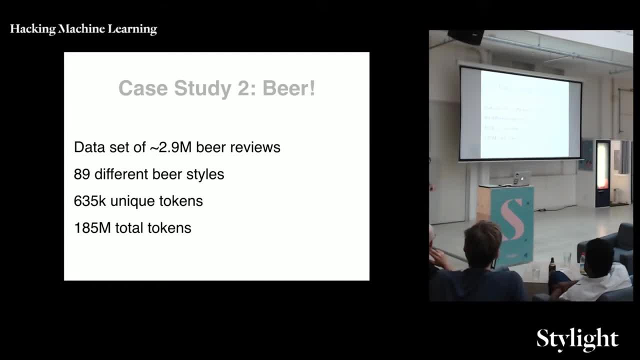 So there are 89 different beer styles And you see the numbers, a bunch of and many, many words in total for this data set. I'm using Doc2Vec in this example, But the snippet looks very similar, So you import the class first. 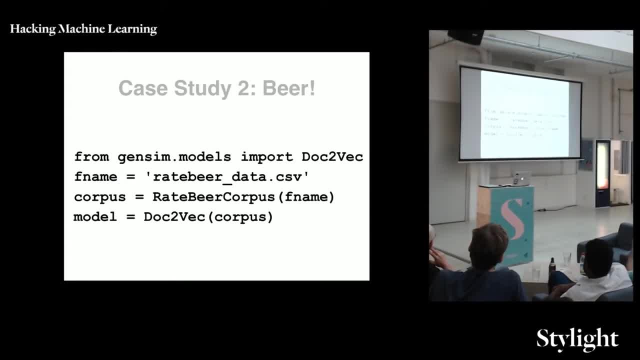 You have your data. This time it's CSV, It doesn't really matter. The third line: again, it will be your custom corpus reader And because we are using Doc2Vec in this case, the corpus reader is a generator that. 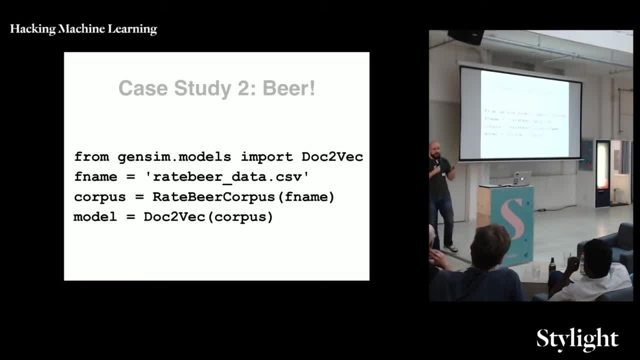 is going to yield one review, together with the beer style as a label. If you remember the probability for Doc2Vec, it has an additional label And I used the beer style as a label. Load it as a model about one gigabyte of data. 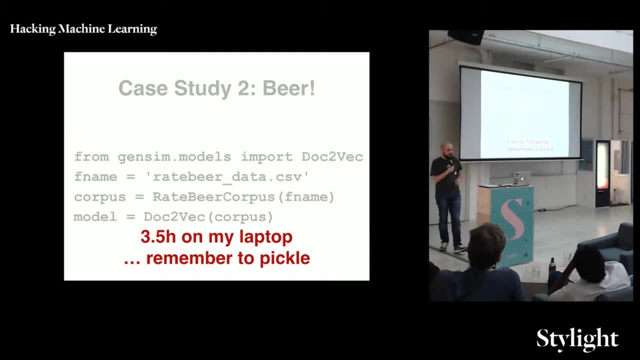 So 3 million documents, one gigabyte of data, approximately 3.5 hours On my laptop. there's a bit of pre-processing So the model maybe takes two and a half three hours. So suggestion is: remember to pickle. 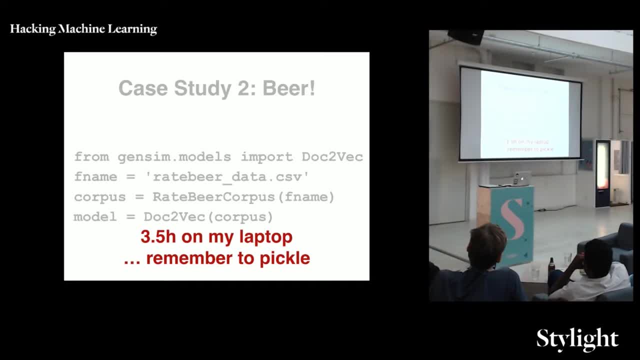 If you close your Jupyter notebook before pickling, you need to waste another 3.5 hours. So now you know that it took me seven hours the first time. So we have document vectors here, So Doc2Vecs, as you see. 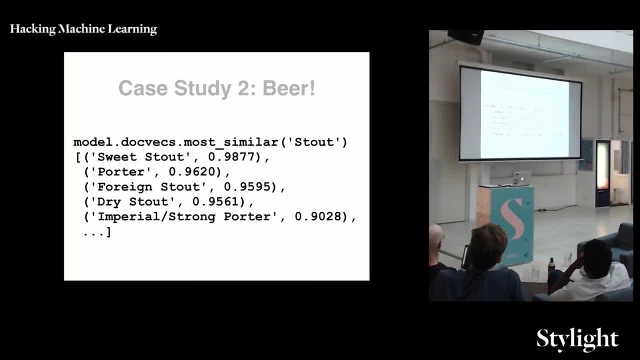 And we're looking for similarity between these labels, these beer styles. So Stout is the name of a beer style, It's a type of dark beer And if you look at the most similar document IDs, if you want, you see different variations of Stout. 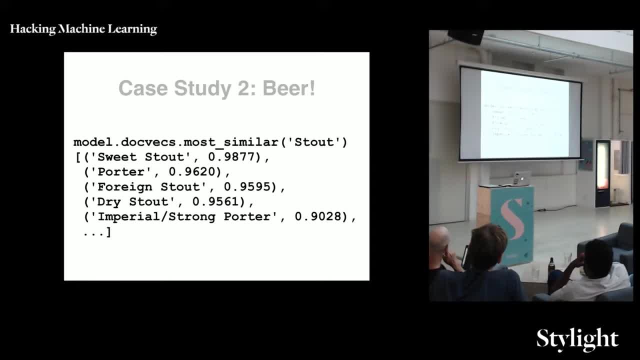 So Dry Stout, Sweet Stout and so on. You see Porter, which is also a dark English style of dark beer, And if you carry on with the list you will see All the sort of dunkel and still dark beers that are less similar to Stout but still they. 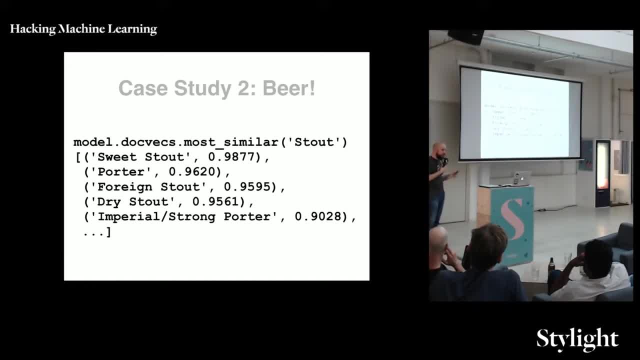 belong to the dark sort of category. So it all makes sense. Once you load the Doc2Vec model, you also have vectors for words, So you still have the Word2Vec as well, So you can check what are the most similar words used. 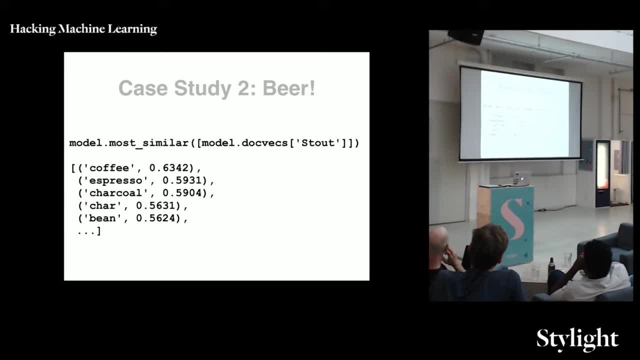 to represent the word Stout. So Stout is dark beer. Aroma should be kind of like coffee or chocolate, if you want. So you will find coffee and espresso as terms used to describe this kind of beer. You see charcoal as well, because sometimes it's 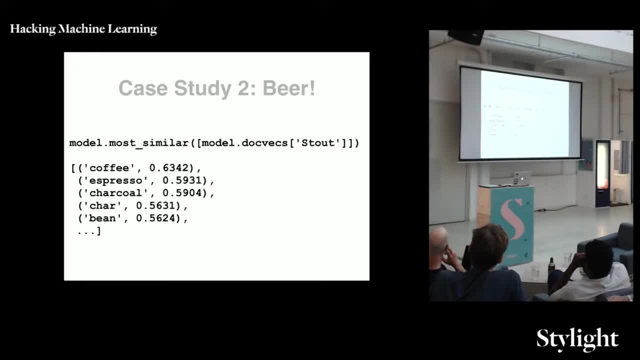 a little bit too much on the charcoal side. So that's also words that are used to describe the beer Bean is probably coffee bean as a phrase. It all makes sense if you know about beer and about Stout in particular. And as a counter example let's say: 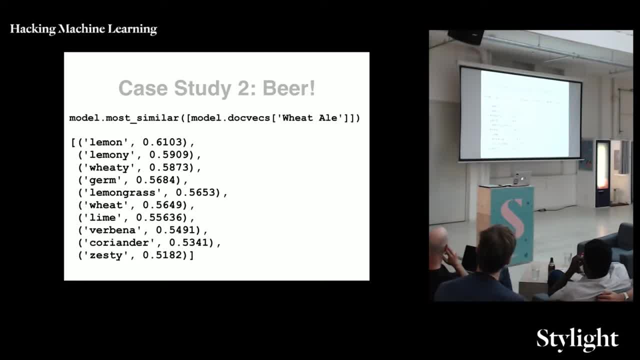 we look at wheat beer, wheat ale. The aroma is kind of like lemony, orangey zesty, So coriander seeds. Again, it all makes sense: Wheat beer. so the data set is a bit biased in favor of American style. 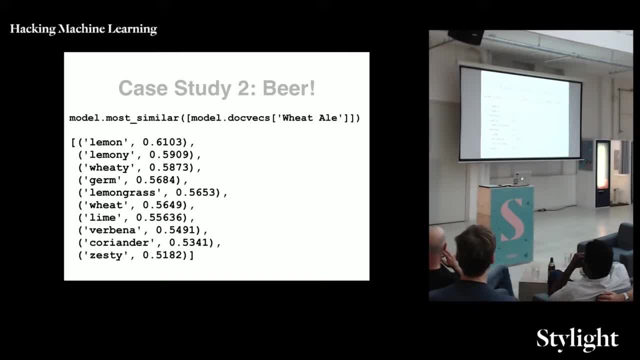 So these are probably American wheat beer rather than Hefeweizen, if you want. So don't get too upset about this. That's just the data. Now we have this- 89 different styles of beer- So I took the vectors. 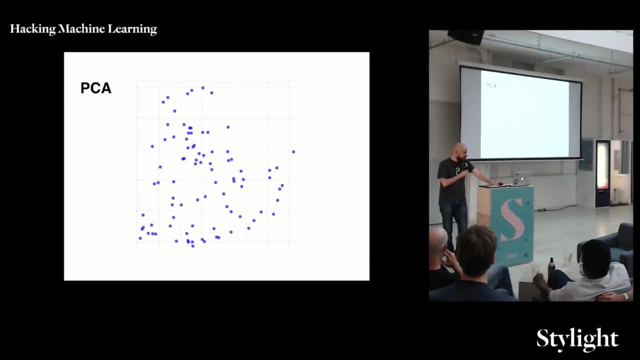 The vectors have a number of dimensions- 300, if I remember well. Throw them into principal component analysis PCA to squeeze them into two vectors so we could visualize the vectors on a screen. We don't have a clear clustering here, but it still makes sense. 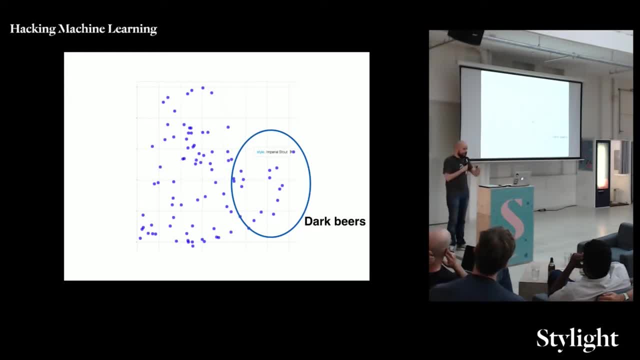 So on one side we have all the dark beers: Imperial Stout, variations of Stout, Dunkel and whatnot. We have all these strong high-alcohol beers together. Then we have the sour beers on different ligues. Bottom left we have all the lagers and pills. 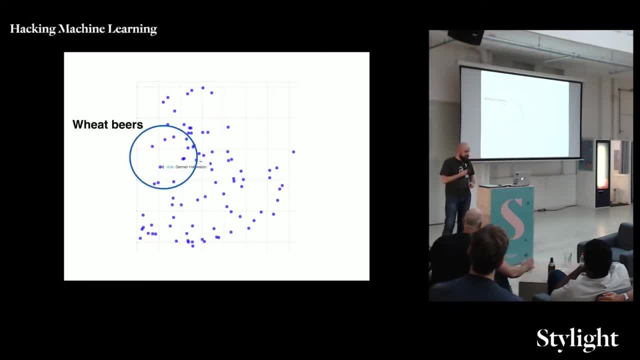 kind of German and Eastern European styles with beer as well and so on. So even though you lose a lot of information when you're going from 300 dimensions into two dimensions, it still makes kind of sense And maybe completely random, but I notice on the X dimension, 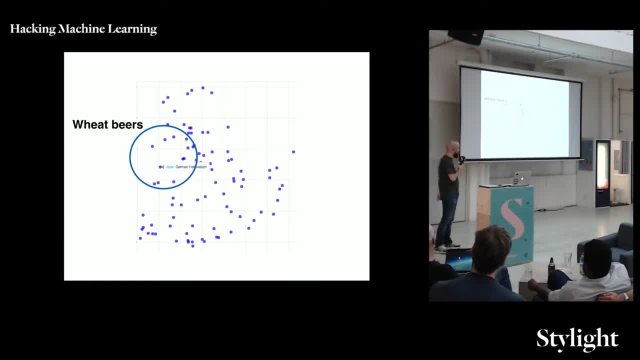 we have the color, So light beers are on the left and dark beers are on the right And kind of brown, orangey, copper kind of colors are in the middle. Maybe it's random, Maybe it's not, So the obvious. 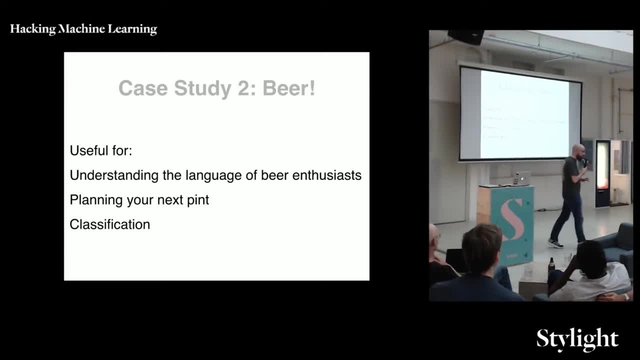 Do you reduce those to, At the beginning, 300.. So each word vector has 300 dimensions As a rule of thumb, not less than 100 and not more than 1,000.. It's kind of a good starting point. 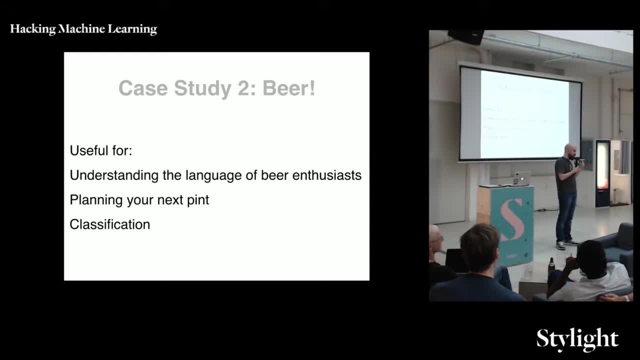 So those are binary vectors of each word. After PCA you have two dimensions, yes, And the choice of two is just to plot it. You can do three and do a crazy bulky. you know everything about it. 89 styles. 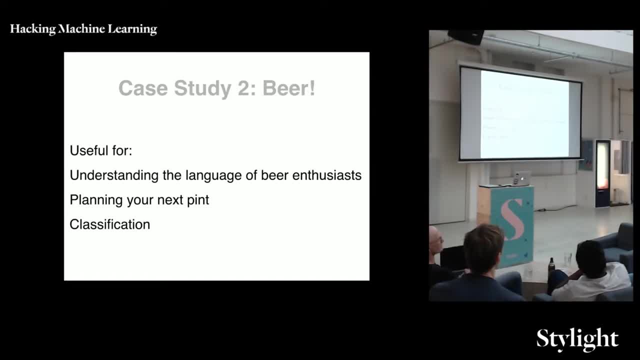 Three millions, Three million. Yes, More on this. later It was a question about complexity. more on this. later, It was a question about complexity, complexity and how it scales, so the well. the obvious applications of this is kind. 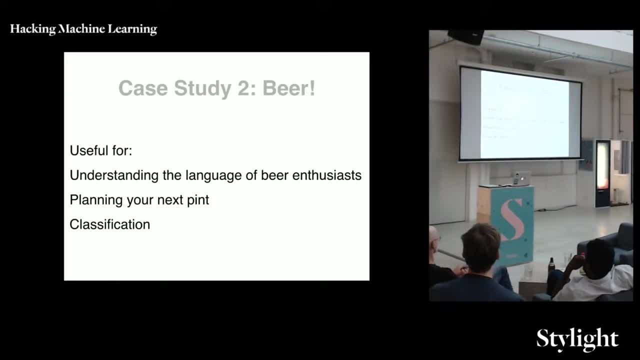 of choosing my next beer, which is the the point of this evening for me, right? yeah, and just as a remark, it's really about understanding your data set. okay, so this is about understanding the language, understanding the bias of the language and so on. it's really useful tool as a exploratory analysis and also. 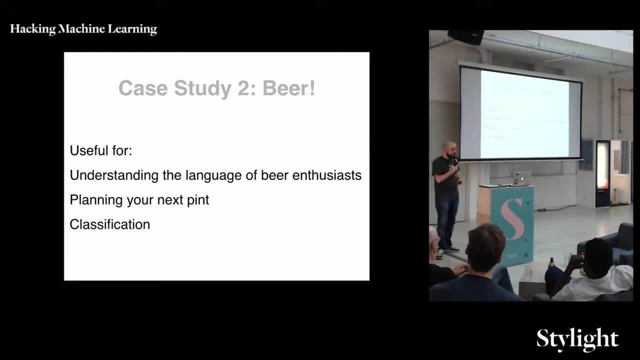 I applied in in classification so comparing to a traditional bag award approach, it was classifying better. so, given a review, can you predict there was the beer style of this particular beer review. using word embeddings gives you slightly better performances than traditional bag awards, as kind of expected. okay, wrapping up, maybe you've seen this before in. 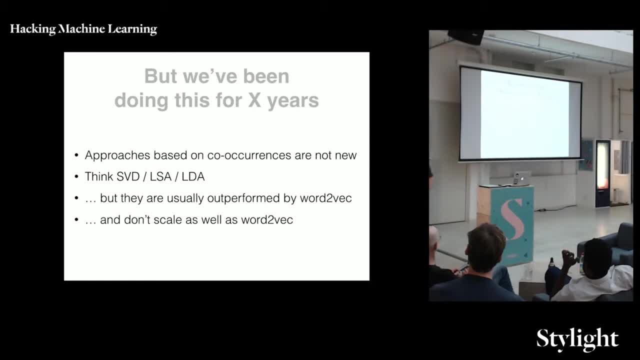 particular in the past, but I think it's really important to understand the particular approaches in general, based on co-occurrences of words that they've been around for a while: distributional hypothesis from the 50s, and then LDA, LSA, singular value decomposition and all the friends. it's true there's nothing new on. 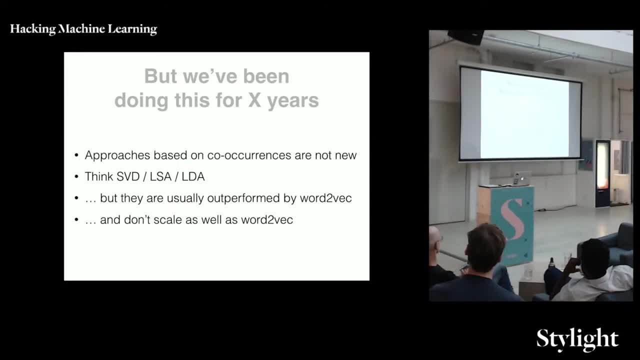 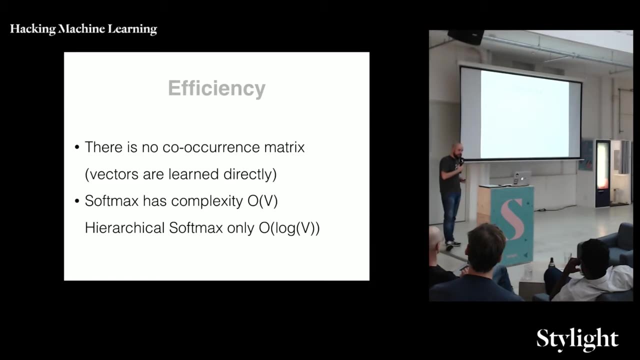 this on this idea. but usually these approaches perform better than the word embeddings here, perform better than other traditional approaches and, in particular, they scale better than traditional bag awards. so I think it's okay, much better because. so efficiency, they're based on co-occurrences, but 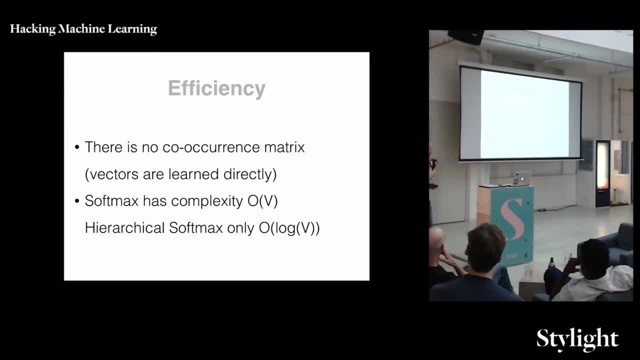 there is no co-occurrence matrix in memory. okay, you don't load the whole co-occurrence matrix in memory. you only learn the vectors directly in terms of complexity. so the softmax depends on you know it's normalized against the whole vocabulary. so linear complexity against the size of the vocabulary and then you 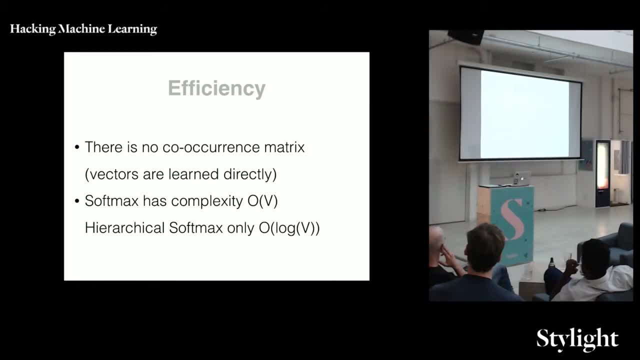 can write. you know, you know a specific set of words. you can write just basically what kind of words are for what you want, so you can have the very rewrite the way you write them. so there's a trick for this, which is called hierarchical softmax, which is also described in in one of those papers that I later. 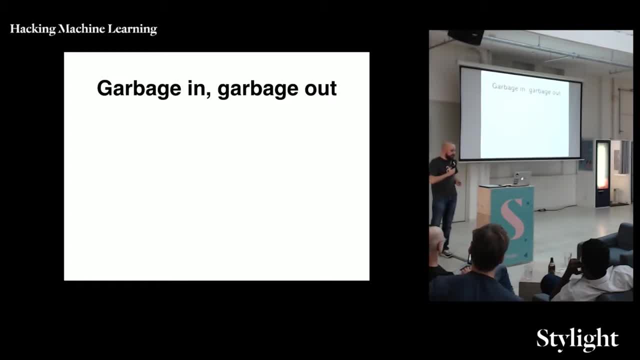 referenced- and I don't remember all the all the details by heart- essentially the sub binary tree as a data structure somewhere. so you go from linear to log badge out. so the quality of your input will affect the quality of your output. So the pre-trained vectors that are given by Google for free, 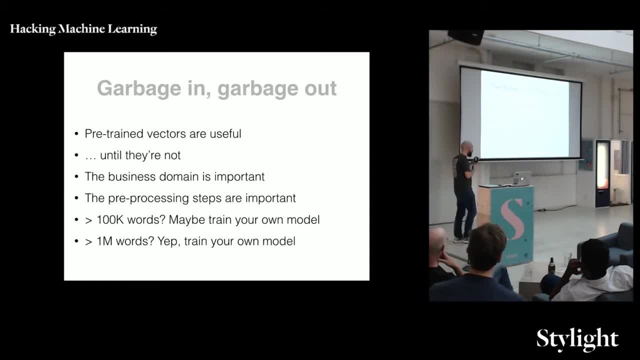 are useful until they're not useful anymore. In particular, the business domain is important, So they are pre-trained on Google News. So we're talking about specific kind of language news and biased towards the US, so US-oriented kind of news. 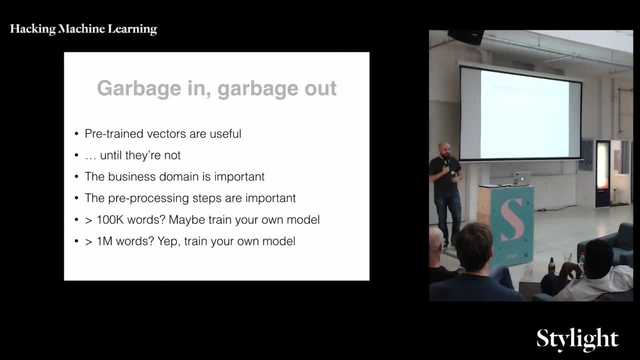 And the pre-processing steps are still important. So what you feed into the algorithm is still important. So the suggestion is: if you have enough data, train your own model. So, as a rule of thumb, 100,000 words, probably you can pick up some of the aspects of the language. 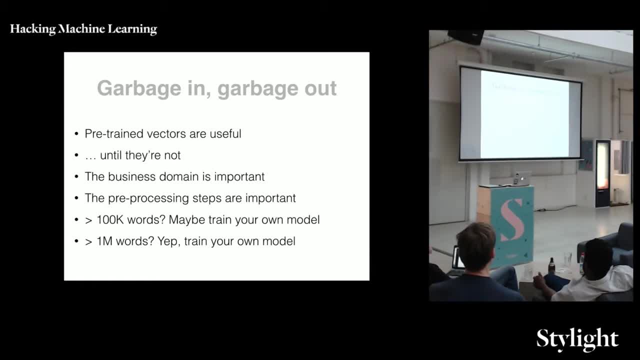 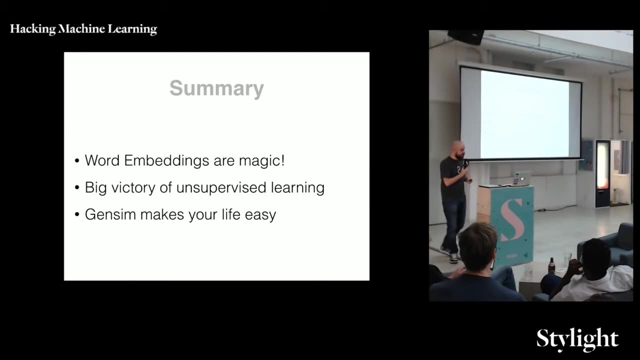 or maybe not. If you have more than one million words, definitely train your own model. That's not a big data set. So that's a generic suggestion for this And just for the end. Just wrapping up. The first time you see these word embeddings. 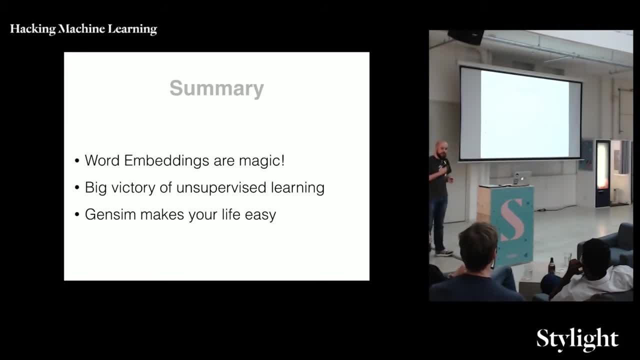 and you do arithmetics, it looks like magic. It's really just a smart application of unsupervised learning, And if you don't care about the theory, I don't blame you. You can just use Python. a few lines of Gensim: 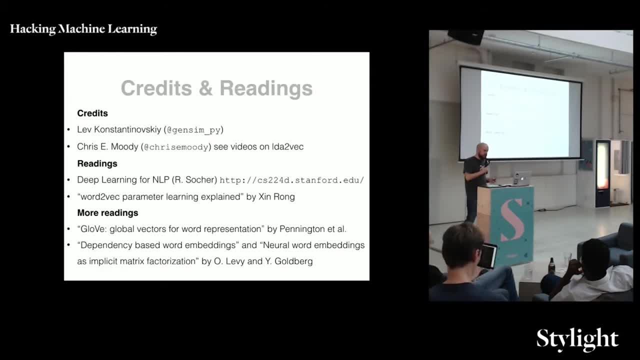 and your life is easy. I just want to reference a couple of things. thank a couple of people. So Lev is one of the Maintainer of Gensim is a friend of mine also. He's traveling around the world, so sometimes he's in London. 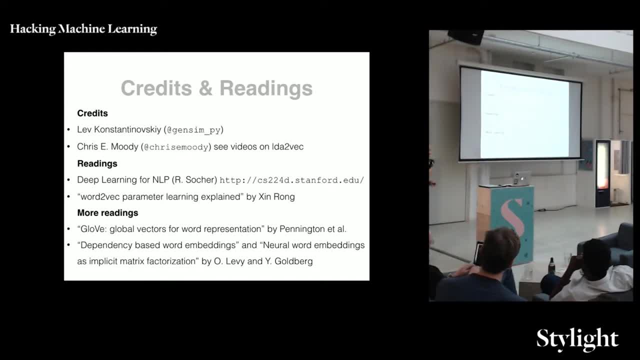 And we've been talking a lot about word embeddings and the work they've been doing on Gensim And Chris Moody. this guy I never met, I've just seen a few of his videos. He has a very nice explanation of word embeddings. 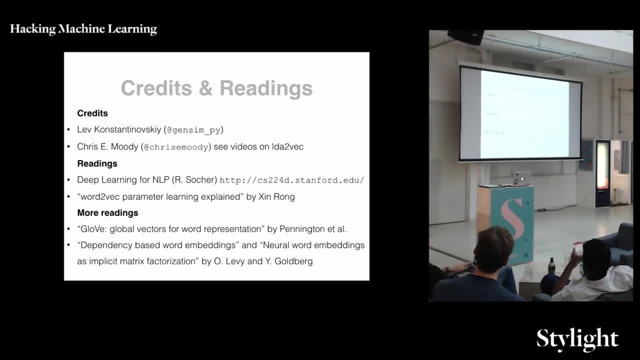 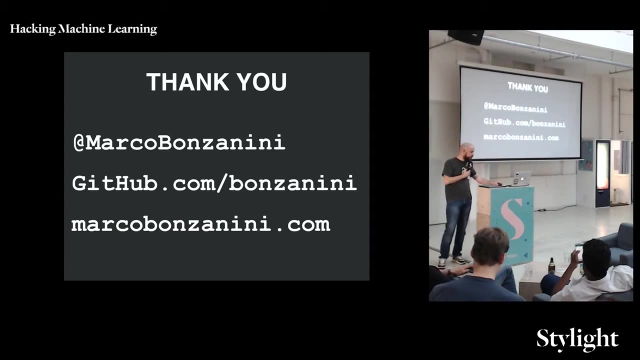 And he has also this joint LDA and word embedding model that he calls LDA2Vec And, if you want to know more, the usual Suspect Stanford and a lot of material online for the Word2Vec. OK, that's essentially closing the talk for me. 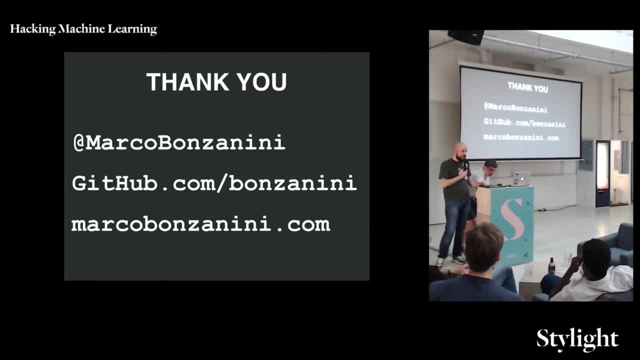 I believe we have a few minutes for questions. I'll be around anyway And I'm easy to find online as well. Thank you, Nice time for questions. Can you give examples for the 300 dimensions And how do you define them really? 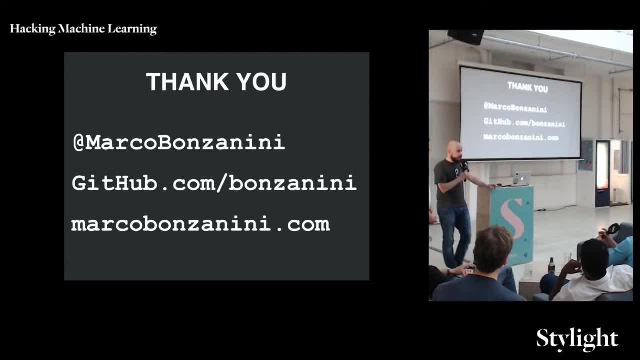 Is that by the algorithm or is there some human interaction? How I define the dimensions? Yes, So the idea is I don't want a huge number of dimensions, so the vectors have. it's easier to kind of handle this kind of problem. 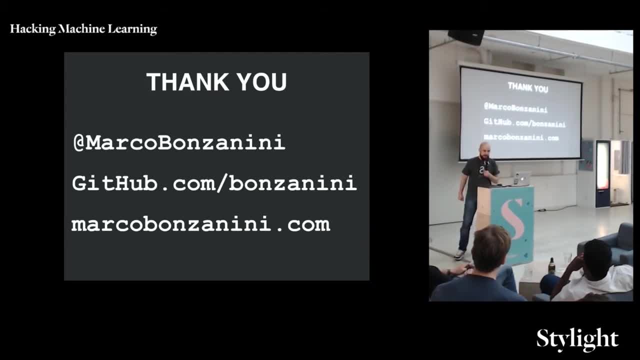 As a rule of thumb, as I mentioned earlier, less than 100 dimensions- OK, Maybe you don't pick up these notions of similarities- And more than 1,000, it doesn't give you more, So people usually start with two 300 dimensions. 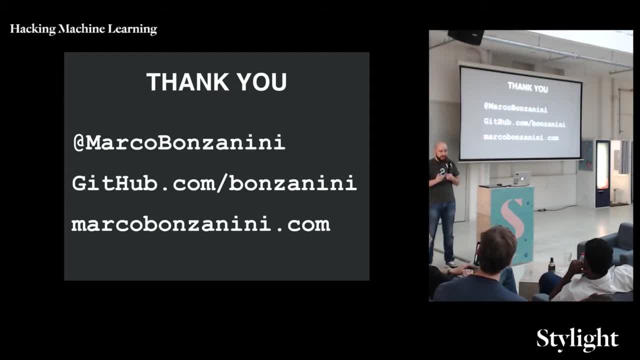 That's an empirical kind of observation. That's what you see in many, many papers, And this number is purely empirical. So you define how many dimensions you want. It's up to you By default. if I remember well, you have 300.. 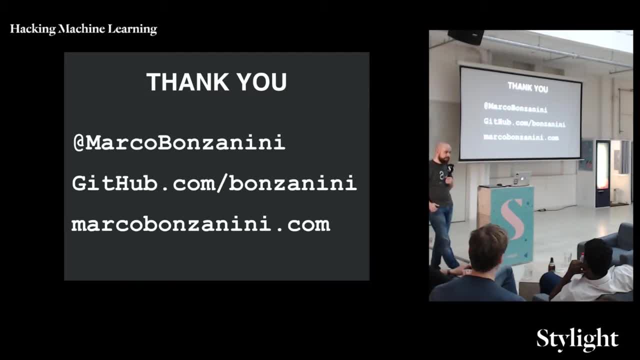 When you pass the corpus to the Word2Vec class, you can define how many dimensions you want. As simple as that. So you take the 300, and you take the top 300 words, and those are No. You initialize the vectors randomly. 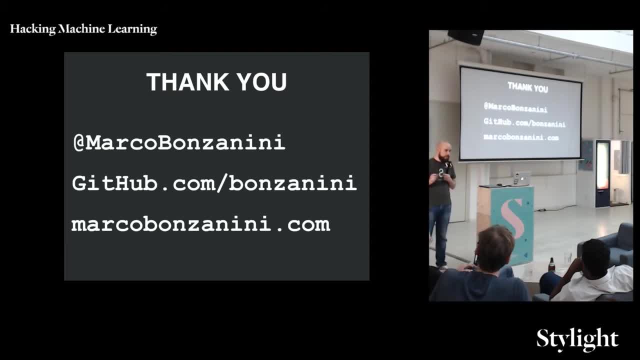 So you have 300 random numbers And then the algorithm looks at the co-occurrences and it will bump up using stochastic gradient descent. So, stochastic gradient descent, It has the objective of maximizing the probability of the context word given the focus word. 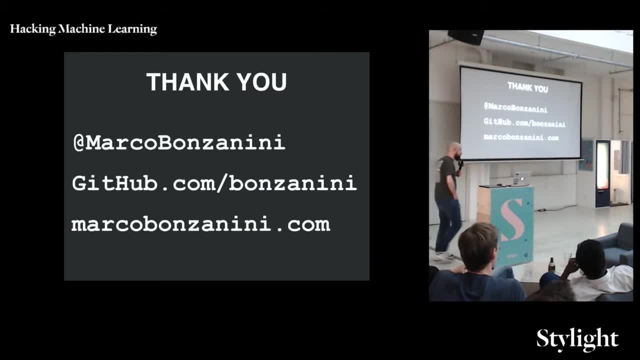 So it's run by stochastic gradient descent. This is pretty cool. Thanks for sharing. This is pretty fun things. So I didn't understand the complexity, only depending on vocabulary size. I have a vocabulary of 30,000 words, which is roughly the English language, but it must depend somewhat. 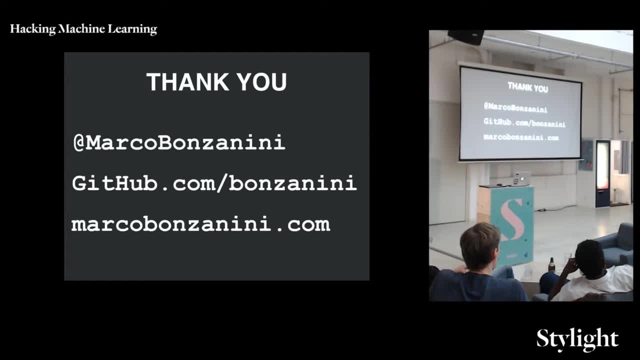 on how many words you're training, right? I mean, it must depend somehow. If you train on 100 million words in the text, that must somehow go into the complexity of how long it takes to train this thing. Yes, on the number of sentences, really. 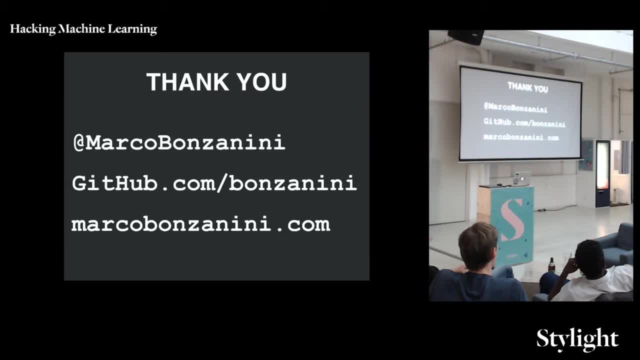 So sentences is how you call the context. It could be sentence, It could be paragraph document. So each sentence essentially would be one of those nested loops. Oh, I see, And then the bigger picture is what dominates really. the story is anyway. 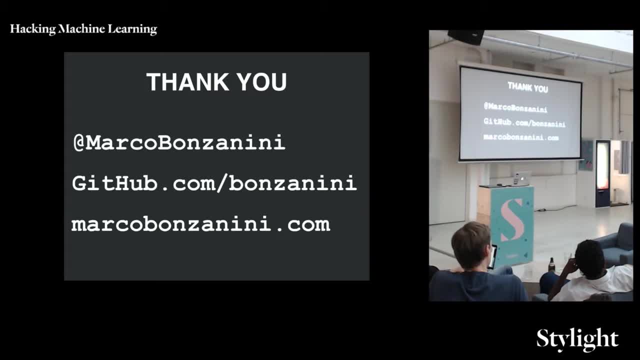 the size of the vocabulary. So a quick other question on priors. How do you let priors flow into this? I mean, if you know, if you have prior knowledge on like I don't know, a beer is related to alcohol. 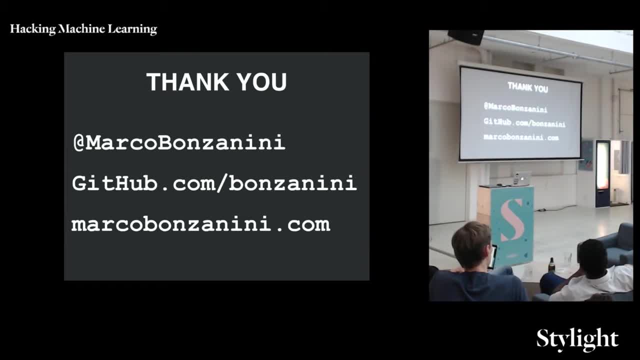 you want to put this knowledge in, rather than- I don't know- let the machine figure it out, Because you know that already. How do you let this flow into your model training? Yeah, you don't. You let the algorithm picking up the language. 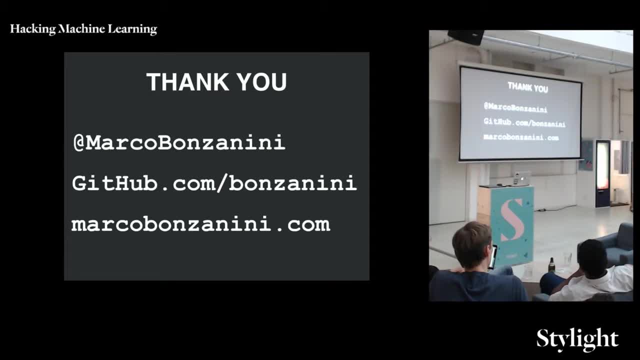 OK, Depending on how the language is used. OK, So you're limited to your training set. You cannot add priors to your model, Which is when I mentioned, when I gave you the example of pizza, and vice versa. So, essentially, your data set will. 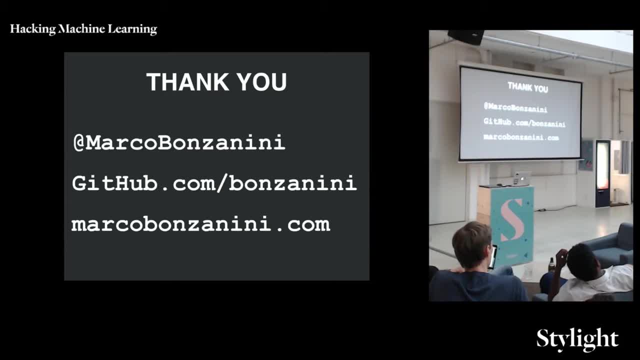 affect the quality of the vectors, of course. Usually the assumption is, with big enough data you end up with these vectors. But you can observe a lot of biases anyway. So in my example I've observed bias towards American styles of beer, just because the data 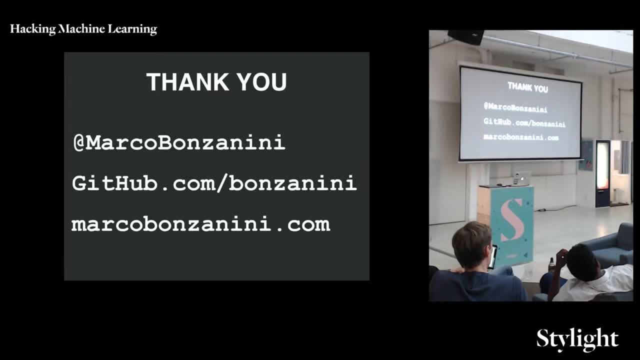 set was coming from an American website. In the Google News example you have certain a bit more disturbing because, say the word for Mexicans? How is the word Mexican used in American news? Usually it's about illegal immigration, right, So the vector is suspiciously closed. 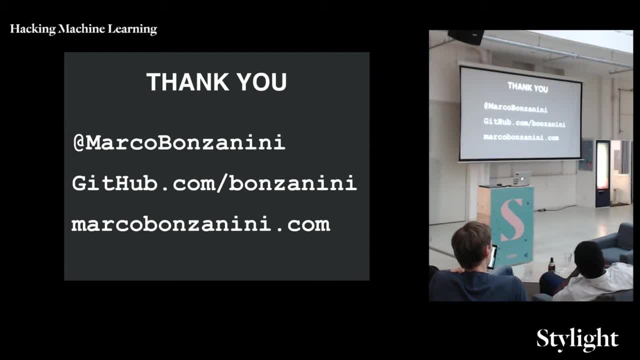 to illegal immigrants, which is a strong bias. And then you observe it also with this analogy: When you do king minus man plus woman is queen. If you do programmer minus man plus woman, you expect to go back to programmer, female programmer. 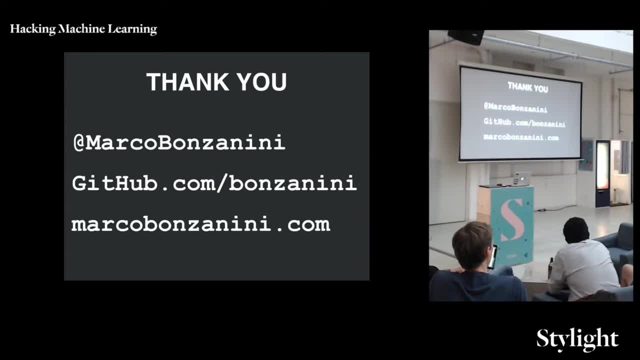 if you want, You don't. You end up with what society thinks should be a job for women. So you have all this little kind of sexist and racist remarks because they're coming from the language itself. So language is biased And the model will pick up this bias. 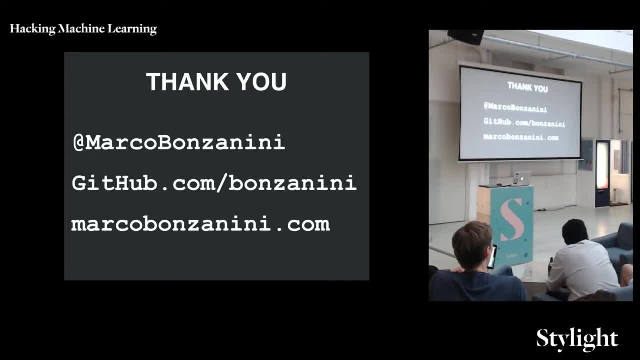 Thank you for the talk. You mentioned on your last slide a comparative model to word2vec glove which I think in the theory is kind of similar but a bit different. Could you comment on the differences and pros and cons of each model, If there are? 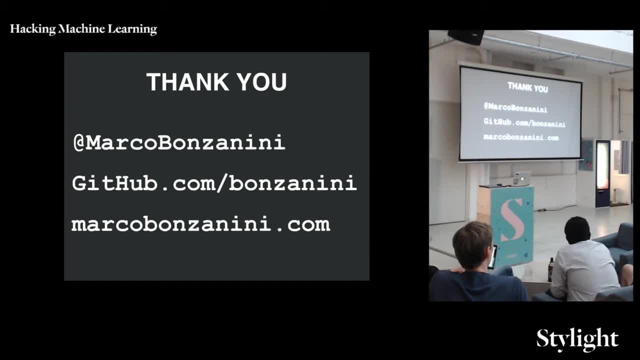 Yes, So glove versus word2vec. I still have to understand it. I still have to understand how they are different. They're kind of similar And for me they're very similar. Maybe I'm missing something as well, But a lot of people are asking the same question. 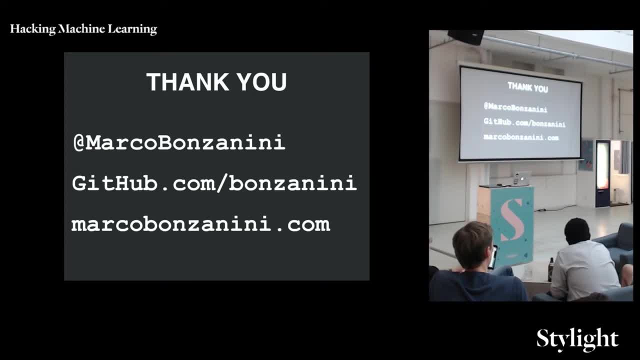 So the short answer is: I don't know, to be completely honest, And I haven't seen, apart from the guys from Stanford who are the authors of this, So this model- I haven't seen any major improvement against word2vec. 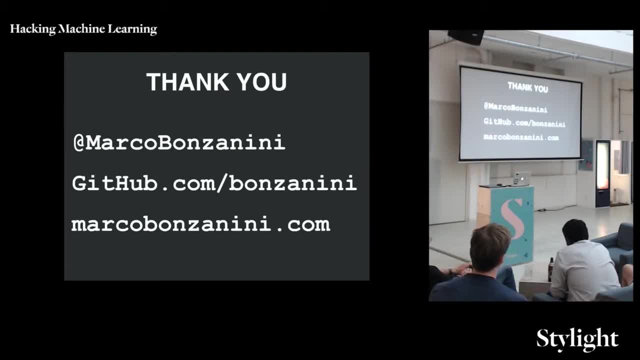 So I don't know. So it's there. I would like to understand. So it's kind of a follow-up work, But I still don't know. Then one quick follow-up question back to the 300 dimensions: Is that decision for 300 more driven? 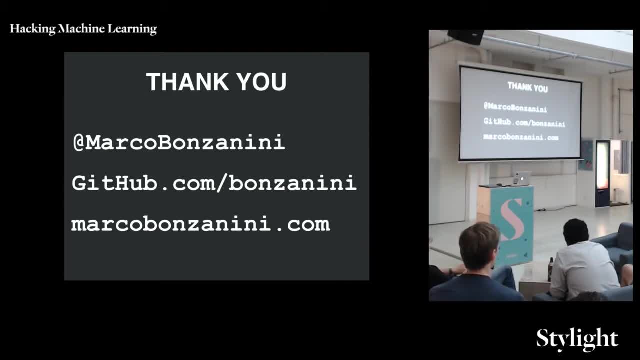 by the size of your data set or more driven by the computational time it takes for a larger number of dimensions or the text content. It's just a rule of thumb, It's just empirical. That's a suggestion that was coming from the authors of the original word2vec paper. 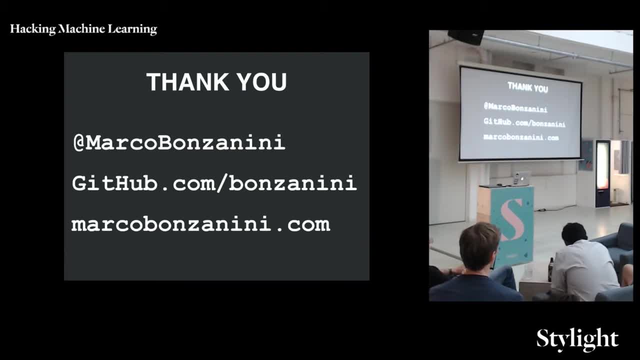 And they didn't provide any particular explanation. They said that we tried many options And the numbers I mentioned kind of make sense. So you start from there And if you like the model, you stay there. basically It's kind of small enough to be the fastest possible option. 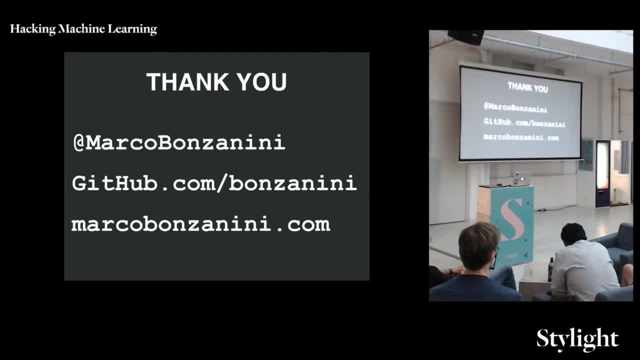 And at the same time it's not a problem And at the same time, big enough to pick up what you want from the language. So purely empirical- I mean essentially- it goes well down to how sensitive you want to have your data set in. 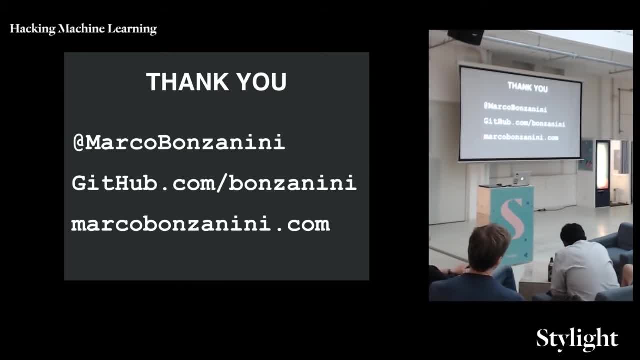 So if you have only one dimension, you basically have only one scale, like from cold to hot, And if you have really complicated text, maybe you want to add way more way basically to compare different dimensionality of different ways, like those words. 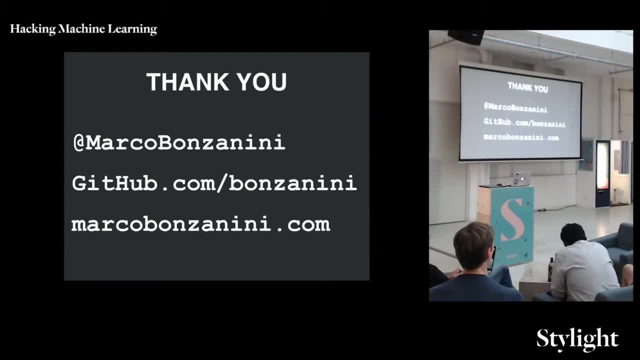 Because eventually you put it in space and you want to compare Or just like a matrix. multiplication that he was showing is basically the same. So if you want to embed more of those, you can do that, But I think there's also too much of those in a way. 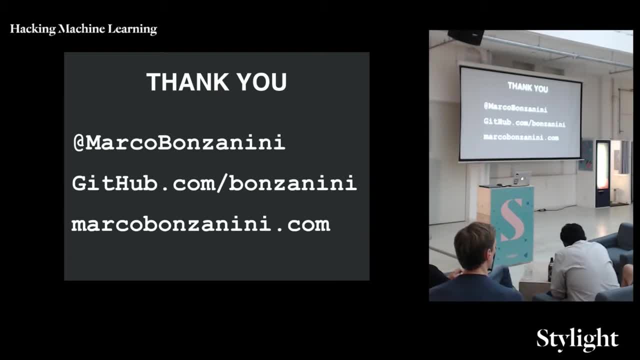 So next one: Some people try to force a meaning on these dimensions, So that there's a notion When I show the initial example: Rome, France and so on. it's a dimension for being a city, a dimension for being a country. 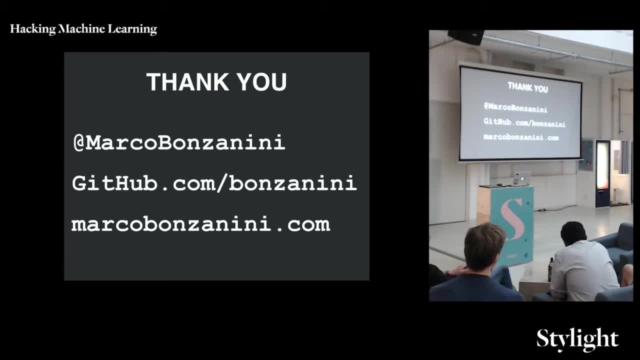 It's not true. So these are just dimensions. They don't mean anything in particular. The example was just made up to the vectors. Find these analogies between them. So presumably you could look at the vectors and you've got a sense of the PCA. 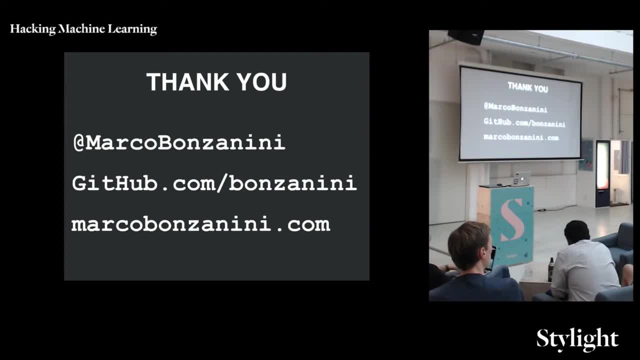 and you might not have to be able to look at the PCA profile and all the interventions. So now we can get an idea about how many you actually need, Right, Yeah, Yeah, I guess you can look at it in this way. In the case of beers, it was obvious to have this color. 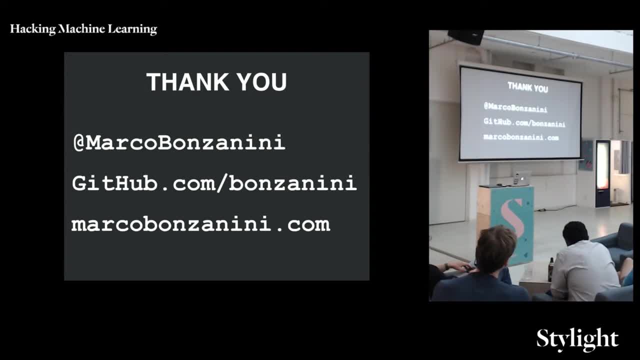 dimension. But is it color or is it kind of toasted malts that are influencing the taste? And of course, Yeah, Yeah, I guess they influence the color as well. Where is the cause effect? It was a side project for me, just for fun. 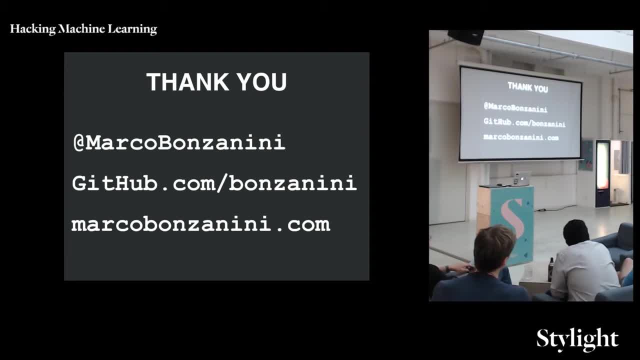 But definitely you can. after you train you can have a look If you're planning to feed your vector to a deep neural network. anyway, how important is still the pre-processing? I would assume if your data set is big enough, the vector or the deep network would already. 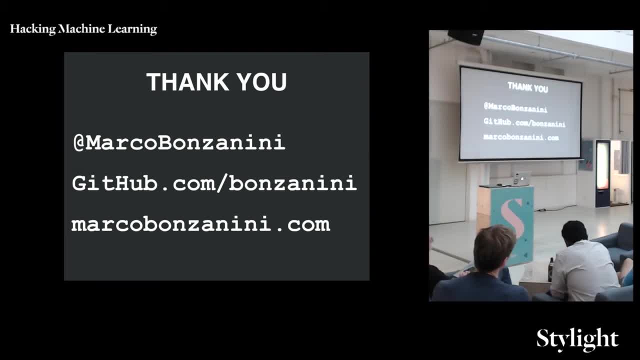 draw some conclusions that Paris is close. It's going to roam in some way, And so is that still important. I guess, like with the position of the word in the sentence, you need to code that in, But otherwise wouldn't the deep network take that job? 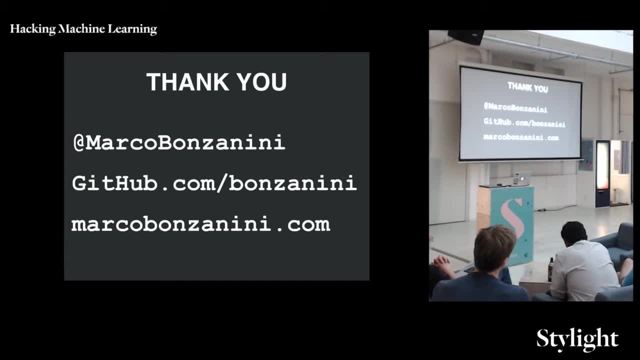 I guess the short answer is: it depends. The pre-processing is important to end up with high quality vectors for words, so to perform this analogy task, And then if you feed these vectors into something else later and you have enough data, maybe it doesn't really matter. 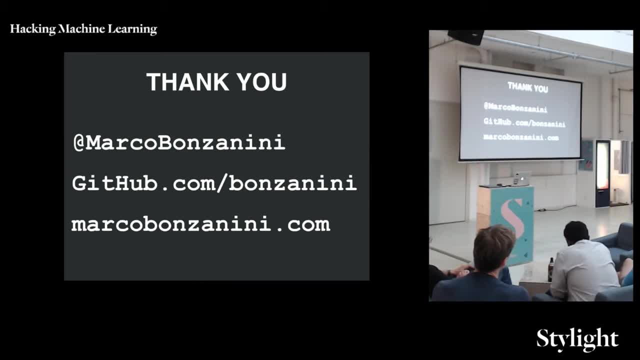 Or if you skip the vector training and you feed directly the text into whatever kind of model you have in mind. maybe it doesn't matter, But what I observe is you have options essentially for pre-processing. So it matters in the sense that you have options. 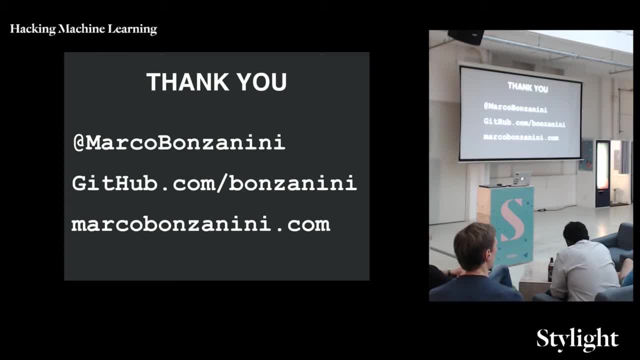 You can choose to do a bit of stop or removal, stemming the usual suspects. You can choose to have ungrammatical sentences and pass only the nouns. for example, With the CV and skills example, we didn't have fluent English. 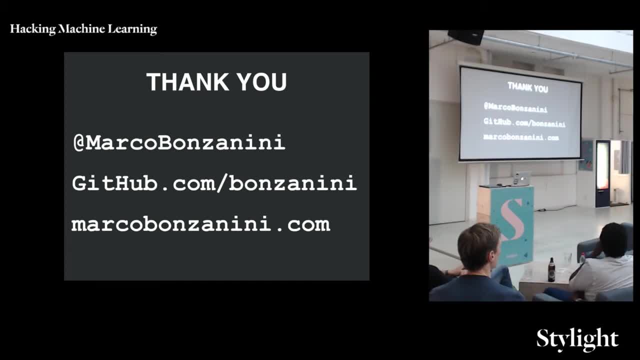 We had a list of skills, So literally it was based on co-occurrences, no grammar picked up whatsoever, So it matters from this point of view, Then, whether it will kind of improve the overall quality. that's to be tested on your data, I would say. 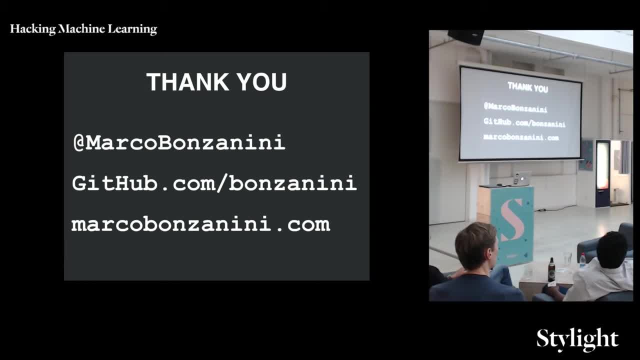 Is there a specific procedure you would suggest for a chatbot? I don't know, I don't know. I haven't developed chatbots. Yeah, I don't know. All right, Yes, I'm back. Hi, Thanks for the talk. 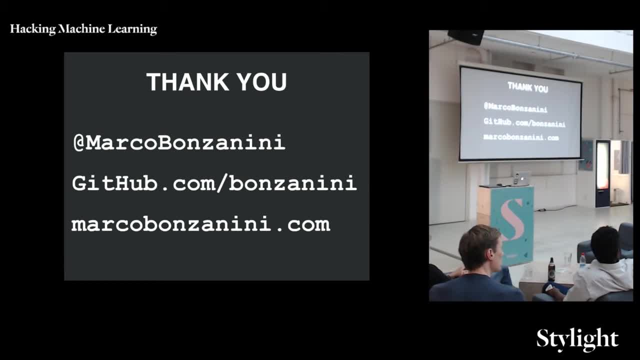 Do the vectors come out of the algorithm normalized, or do they have the same length or do they have different lengths? Are the vectors, sorry, Normalized or are they different lengths? the vectors: No, the number of dimensions is fixed. 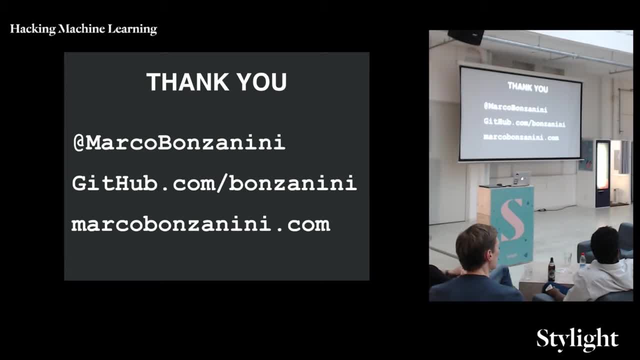 No, but the length of the vector, Like the norm. Oh yes, It's all. the dimensions are essentially between 0 and 1. But do they have the same length? So if you have two words, do they have the same length? 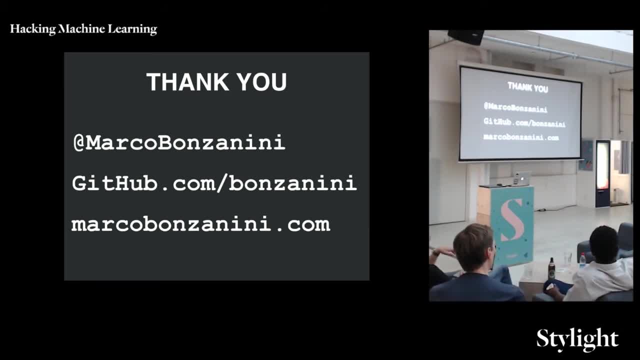 the vector, or is it So what people do? usually they merge. So if you want to model a phrase, you kind of create a special token of word 1, underscore word 2.. Is that what you're asking? No, I guess. 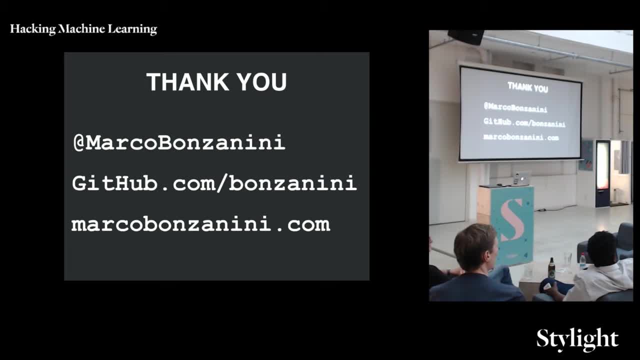 I mean, If you look at the mathematical object of a vector, it has a direction and a length, And are these vectors all the same length and just different directions, or are they different lengths and different directions? I noticed that when people try to compute the similarity, 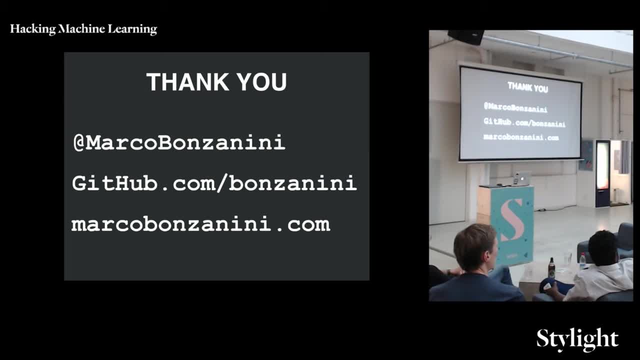 between words: they first normalize the vectors and then do it, So I guess they are not normalized before. I'm not sure I understand the question, so maybe we chat a little bit later. Yeah, OK, That's a question, Maybe last one. 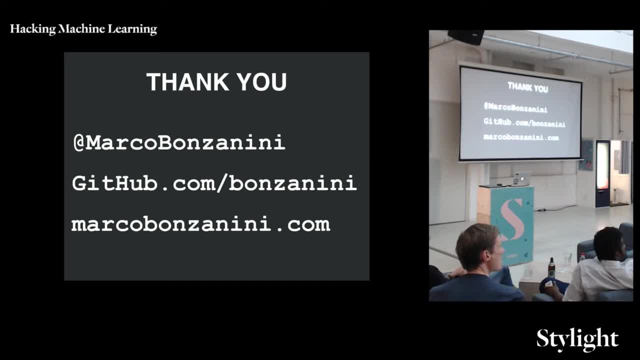 No, OK, One at the back. I cannot see you. You're like behind the wall. I'm bringing that. I have three questions for you. How big was the memory footprint in your RAM So while you were computing with that metrics? 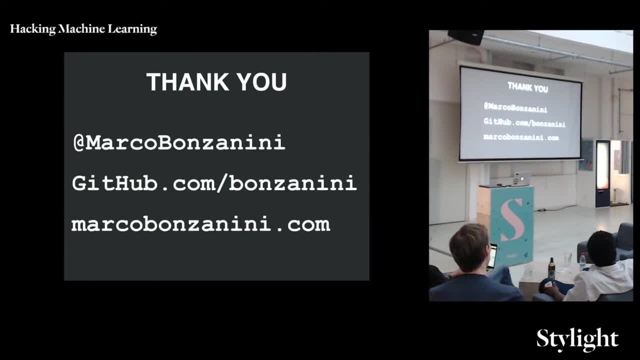 The memory footprint. Yep, I wasn't checking the memory footprint, It was fitting. It was fitting in memory on my laptop. The data set was the bigger one was about one gigabyte, so nothing huge. The output is about 150 megabytes from one gigabyte. 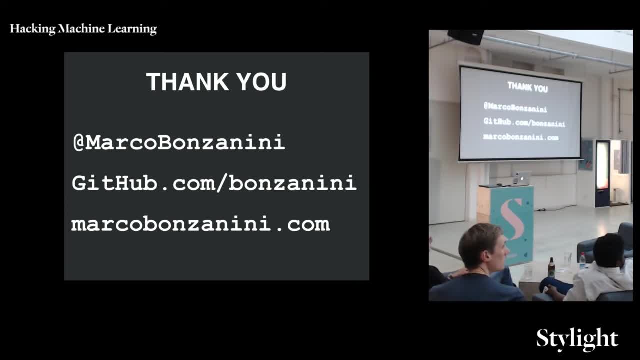 of text to 150 megabytes of data. OK, So when you're saying the output, so were you able to save that output for some later computations also? I'm assuming Can't hear you. I'm asking you. Ah, When you computed that metrics were you? 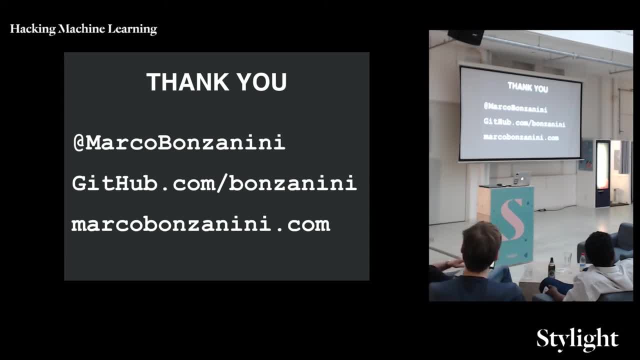 able to save it offline, For example. you don't have to compute next time when you were, let's say, planning to play with the data. So, first thing, there is no metrics computed, They're just vectors, And you can persist the model and then 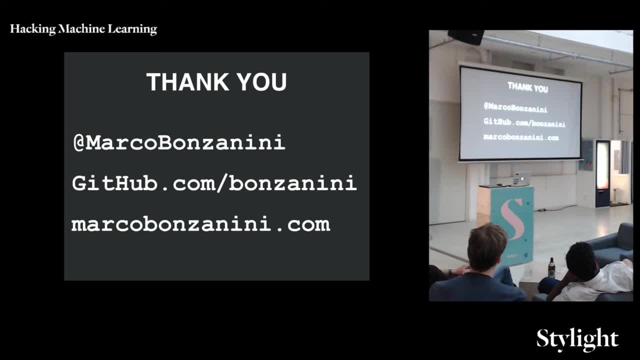 continue the training later. You can add more data later on and it will, in theory, improve your vector representation. Thank you, It answered my third question. Yeah, Can I retrain? Yes, I can retrain. Awesome. The last last one, no. 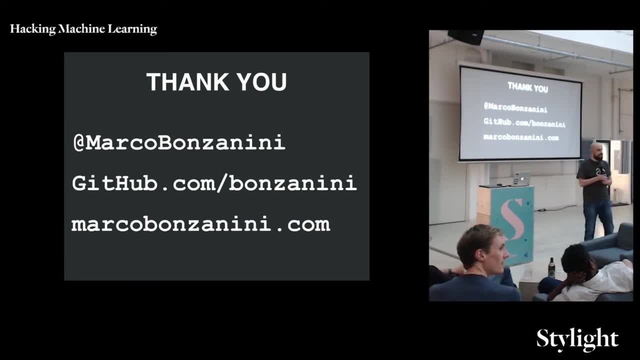 OK, Here's the winner, And after we're having a break. So I'm interested in the work to sentence stuff. Sentence to vector, you know, Yes, Do you have to predefine the number of words in a sentence you want to match, like with a big example of wheat stout?